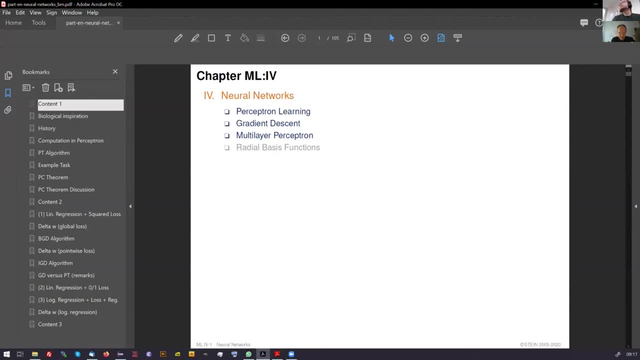 Hello together, good morning, and I hope you feel well. Martin or Michael or the other PhDs or technical assistants, please interrupt me whenever there are things which I should, in addition, mention or there are important other things. I learned, for instance, yesterday from Michael that we have a competition in the leaderboard already. I don't know whether you want to give some details about this, but we will quickly discuss this later. Yes, Yes, Directly after the reading. Is this correct? Yep, Very good. 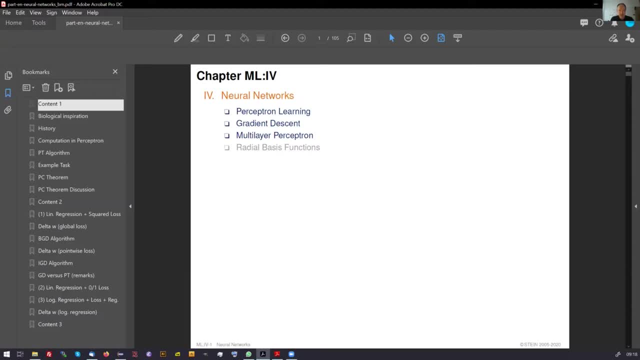 Okay, Today's reading is a short recap of the perceptron learning algorithm which we had, a short recap of the gradient descent, an explanation how these things fit together, and an extension to multi-layer perceptrons, which forms the basis of all bigger neural network architectures, including deep learning, which we have today. 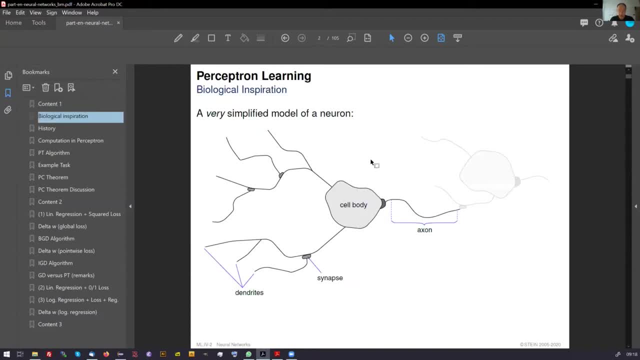 Last week I started with a slide like this, where I showed a very simplified model of a neuron, and I repeat this only to emphasize that I want to call it very simplified. Please take this with you, This idea of the biological means inside of ourself or other beings. 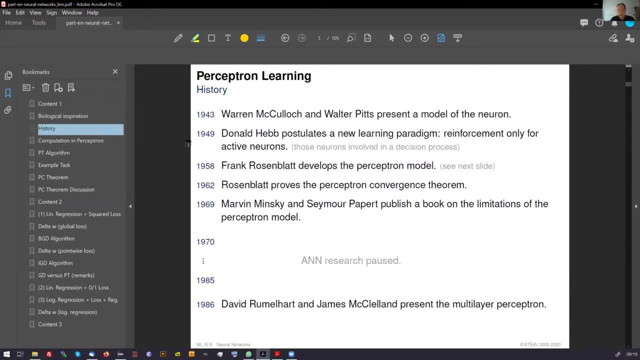 led to an interesting run- how to develop algorithms that learn- And today I will especially discuss what happened here, namely that research didn't continue because of the obvious shortcomings of the perceptron algorithm. However, the perceptron algorithm still opened a lot of doors. 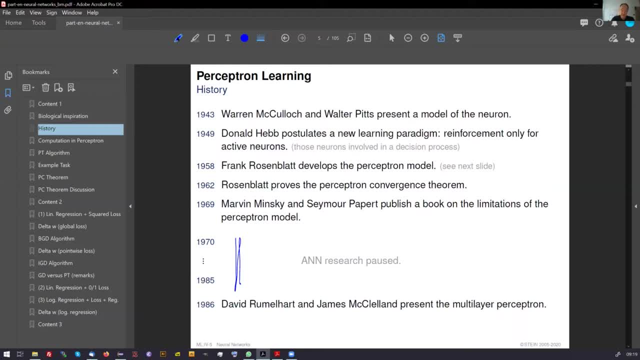 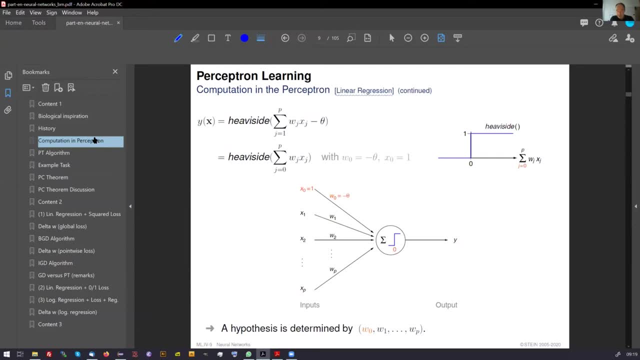 The area of complex neural networks. regardless of this problematic situation, The computation in the perceptron is quite similar to what we saw when we did linear regression. We formed the linear sum of our inputs with weights and compute some output, And while we used the sine operation in the linear regression, we will use here the heavy side. 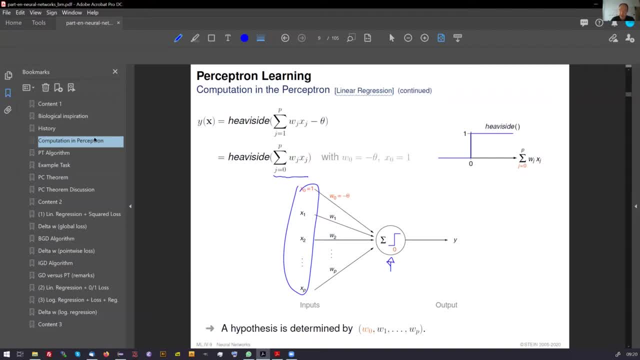 The difference is not big. The sine distinguishes between minus 1 and 1, and the heavy side between 1 and 1.. I emphasize this to show that the heavy side is nothing complicated, has no magic inside and does not make this happen here. 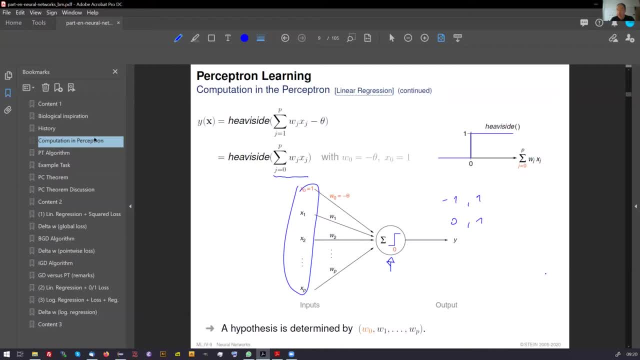 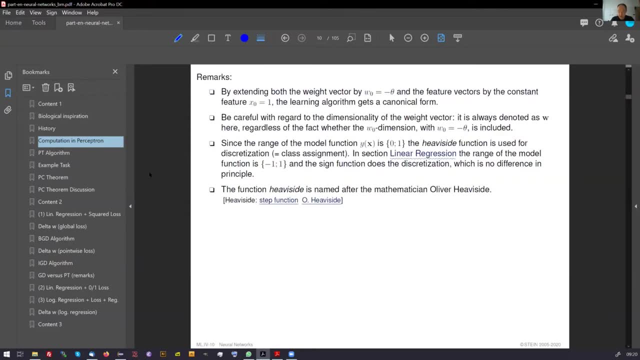 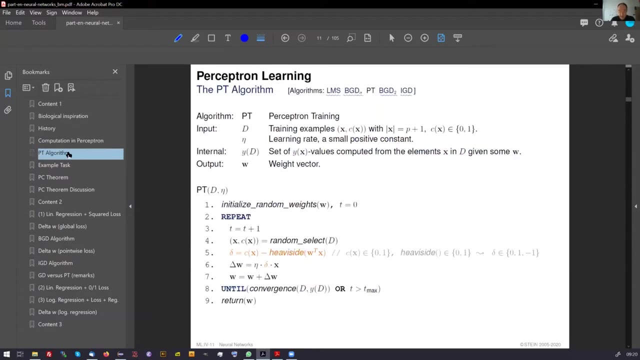 It is only the, the discretization function, which we use if we decide between 1 and 0. I have also mentioned this here again. The PD algorithm is in that sense, not complicated. It has an update rule which compares the truths with the heavy-sided output and then does something, namely something very simple. 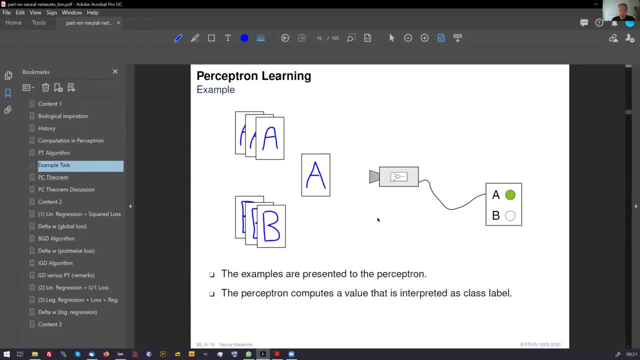 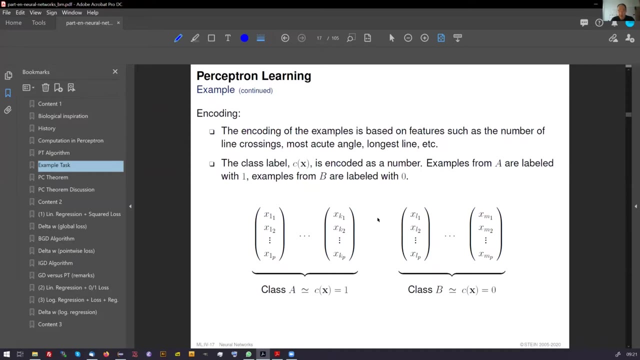 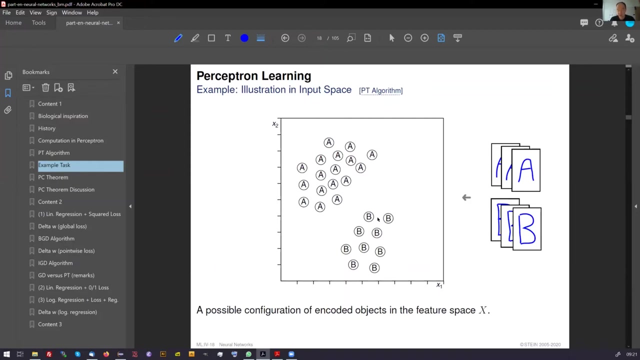 I illustrated this with a task where we had to distinguish between two classes, here represented as two letters, The letter types a and b, which we might characterize by simple features which we then see in a two-dimensional or higher-dimensional room. I have shown only a two-dimensional room for illustration purposes. 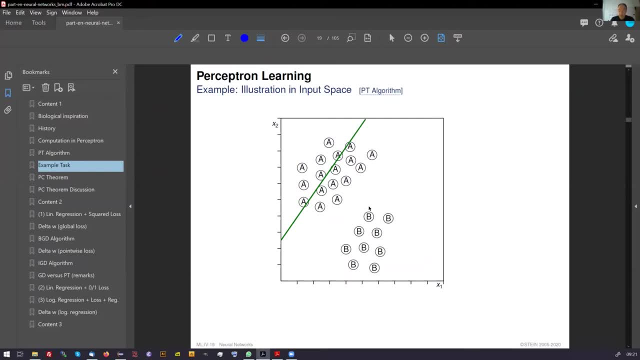 And here is now a separating line. In fact, it's at the moment not separating And we now test examples like the a which you see here, And if it's on the wrong side, Then something happens with a weight vector And it's updated. 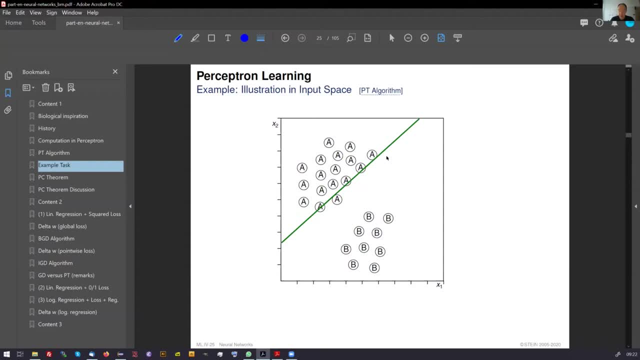 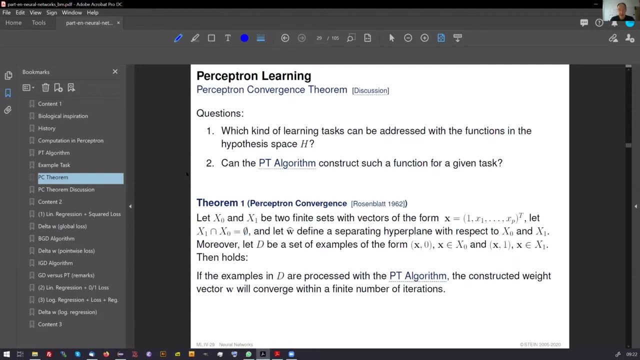 And if these two classes are, it's called- linearly separable, the algorithm finds the solution. The two questions which we show here address exactly this point. What can we do with this algorithm? Namely, find linearly separable. 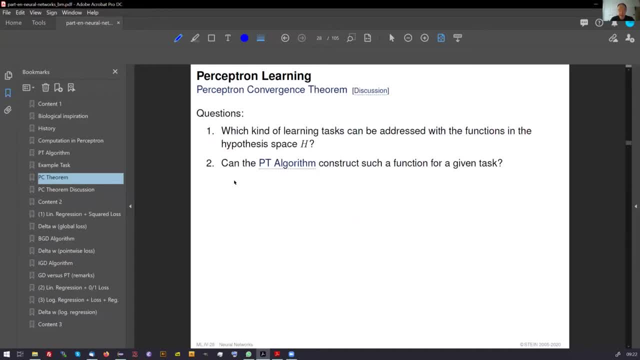 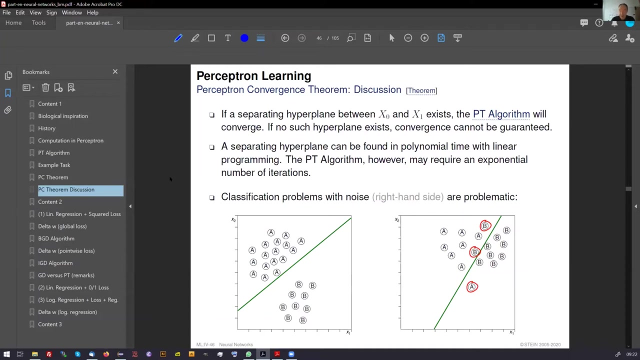 Separable classes. And does this work always? Yes, it does work always, If we can find such a line And the convergence happens within a finite number of steps. If such a hyperplane cannot exist because the classes are not linearly separable, 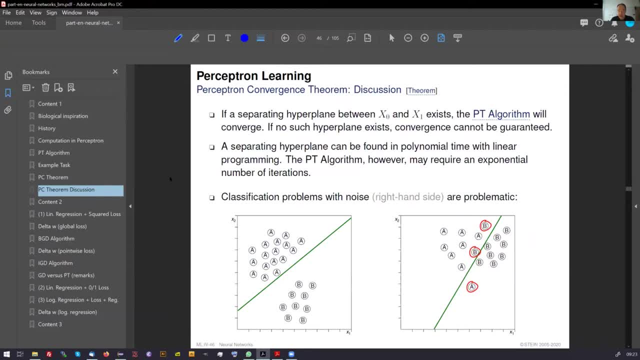 Then we have a problem: The algorithm will stuck somewhere And cannot come up with a solution. And we saw already in earlier times that with linear regression we can produce a solution. And you see the situation here. We have this line And regardless how we draw this line, 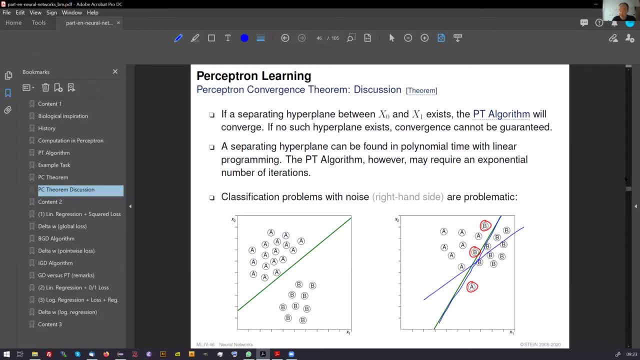 There will always be misclassified examples. And here is an interesting thing: There are two answers on this. How to copy this? The first is to use a regression with gradient descent, And this can be a complex regression. The second is to develop more complex architectures. 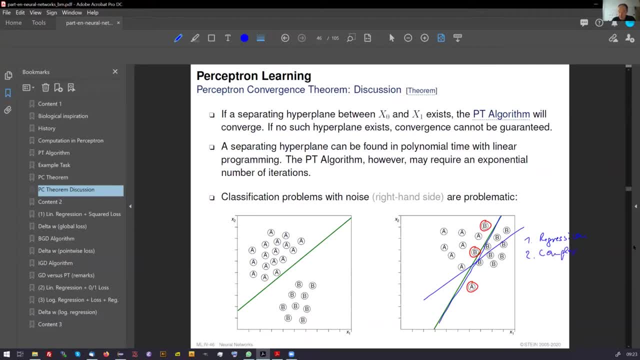 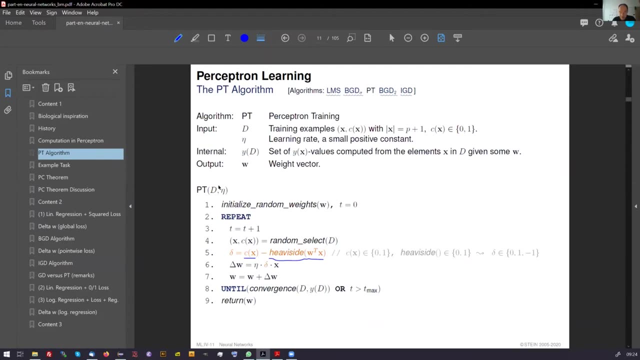 Just a quick interruption, Benno. There's a question in the chat. Yeah, And it says: how does sigma in the perceptron Learning algorithm have a range minus one, zero one? So Sigma, Where is sigma? I think the error. 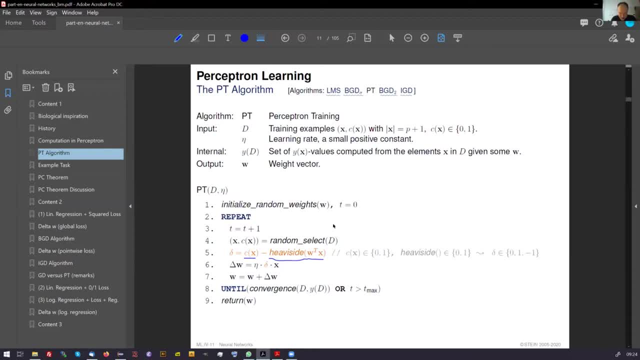 Delta is what it's meant, Thank you. What is the question again? Does the delta have a range between minus one zero and one? Ah, yeah, We can check this. We have. Perhaps this is wrong. I will see this. 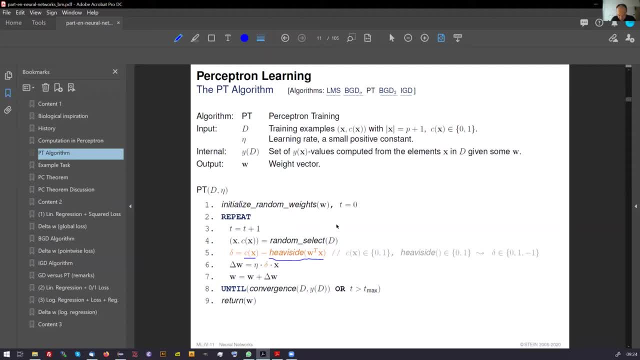 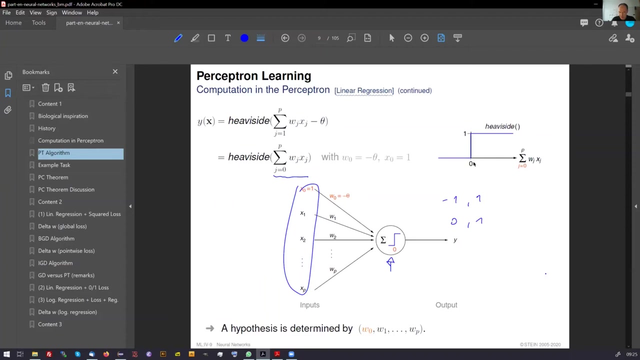 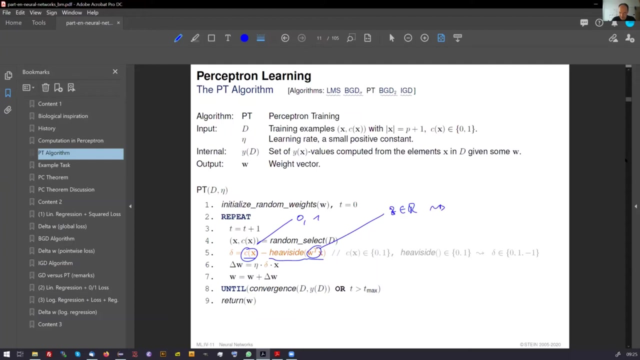 No, I will directly see. Our classes are zero and one. Here This product gives something, Here This product gives something. And if it's larger than zero, this product Heaviside outputs a one, Otherwise Zero. And now we have. 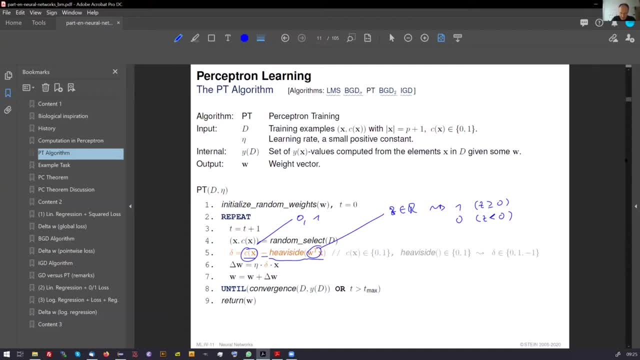 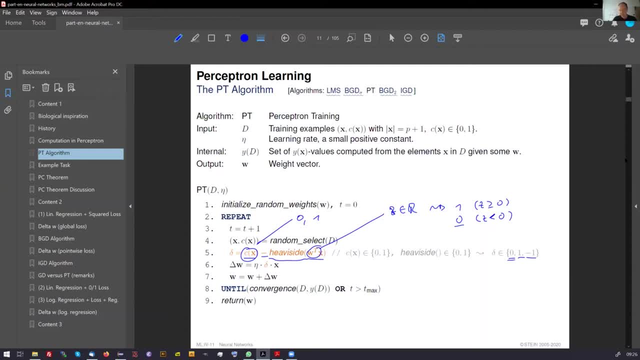 One Minus One Minus One And one minus one gives zero. These are the possibilities which happen. Answer this a question? It does. Yes, If you have a better answer or can they explain better, please say you're welcome here. 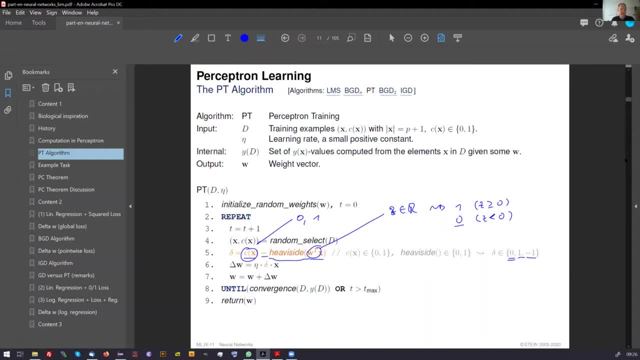 This helps also me. It helps Okay. Okay Now, Yes, Okay, And if you think the things are not clear because I didn't present them properly, please you interrupt at any time. okay, Okay, but you said it's done. 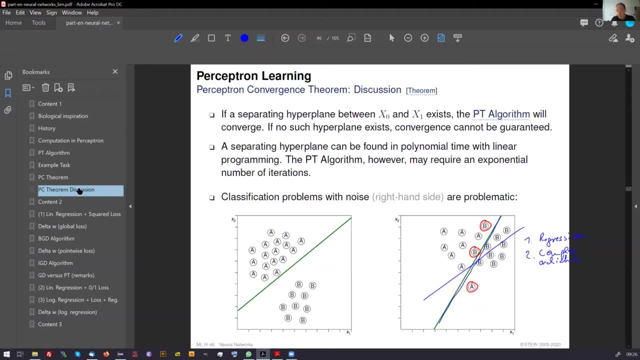 We were here and they can give two answers on this, on this problematic situation. namely, we can use the kind of regression that we pay for this non-correctly classified examples with a loss offset, or we can bring a more complicated line. And both answers are important and are valid and both answers are given. 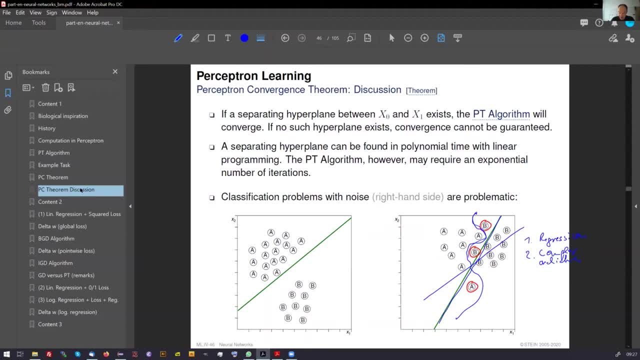 The answer which I show you here is the answer, The answer which we give, for instance, this basis expansion and logistic regression, which we give this support vector machines and which we could give this more complex neural network architectures, The answers where we 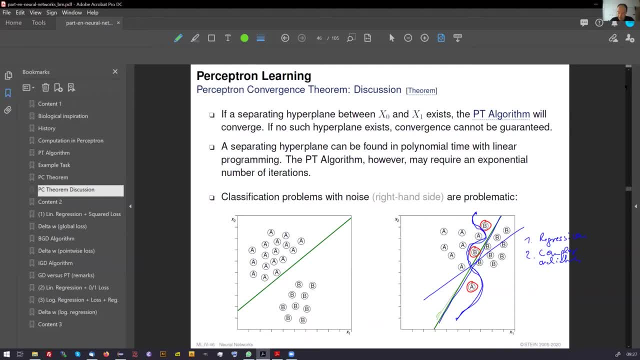 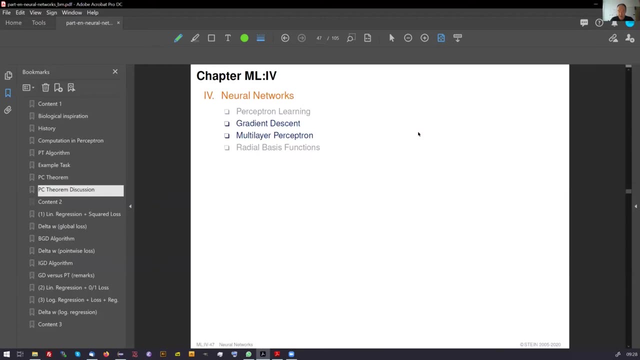 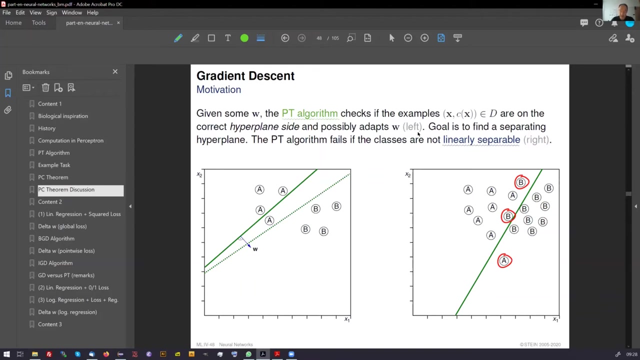 Okay, Draw a straight line. pay something for the misclassification they are given with linear regression and the classical logistic regression. We have developed slides to show you this important difference again. The BT algorithm works only in the input space. It takes, for instance, this example: 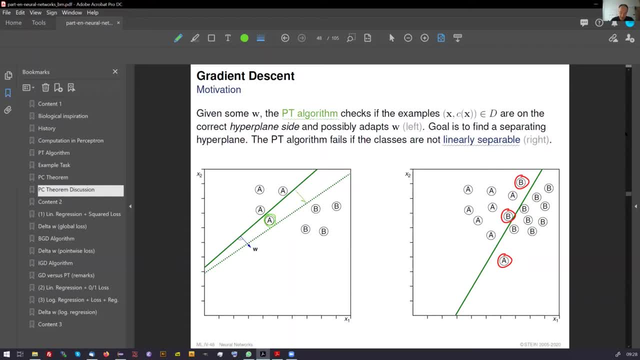 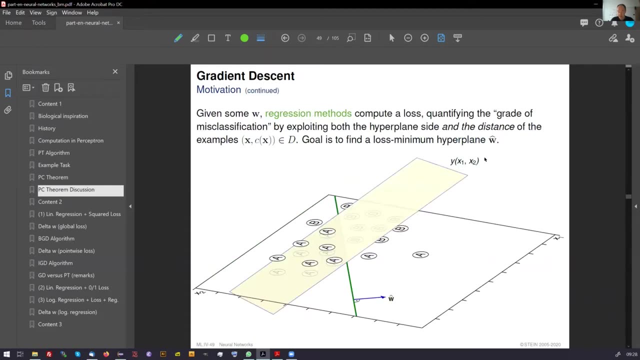 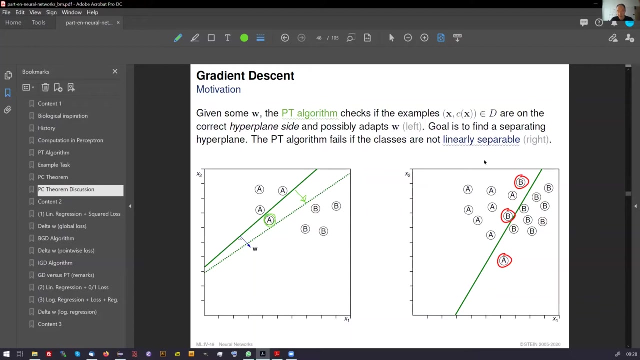 Turns out it is on the wrong side and goes here. The support vector machine, which will come next reading, does something similar. Regression on the other side looks at the global loss. That means it does not look only into the input dimensions but into the input output. 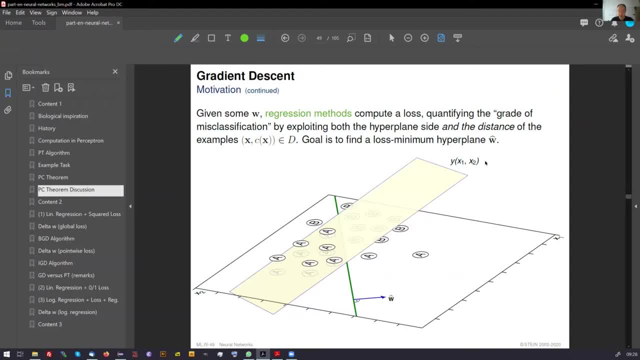 space And for those elements which are wrongly classified. you see, here we see a residuum And from this residuum we compute a loss. And the big difference is to Okay, Okay, Okay, The perceptron algorithm, that this loss is dependent on the hyperplane distance. 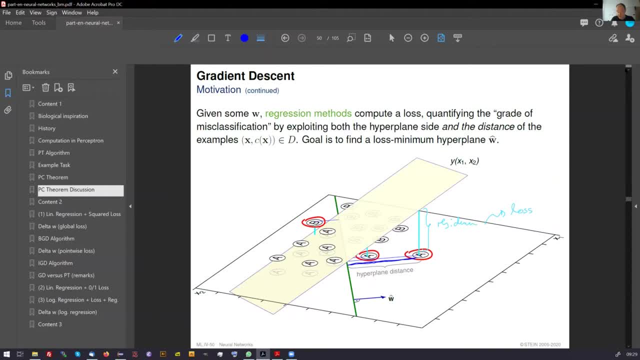 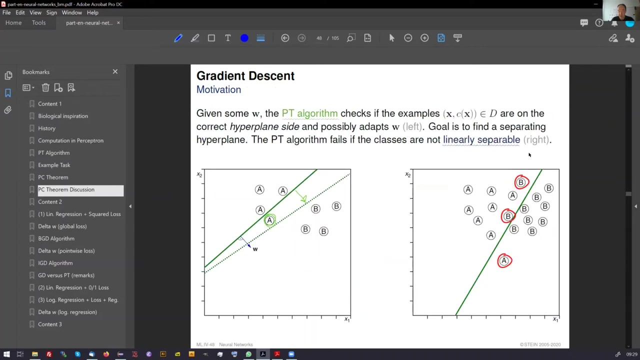 The farther we are away with our misclassified examples from the hyperplane. that means the grade of misclassification of cortis. the larger this is, the higher is the loss. This information, Okay of the hyperplane, is not exploited in the classical perceptron algorithm. 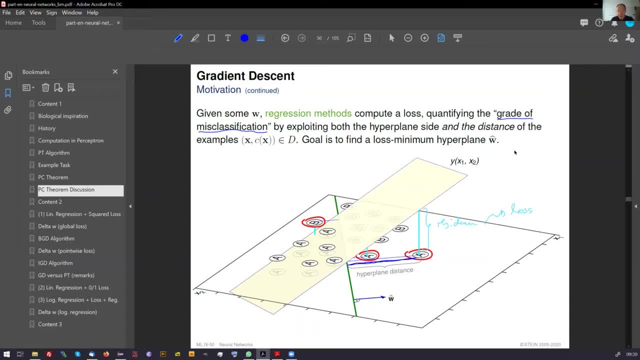 Gradient descent now is a method to compute this loss with an iterative algorithm. That's all. We can do this with other algorithms as well. but gradient descent has a few advantages, namely it's robust. it can be easily adapted to large datasets. it has also the deficit that it has convergence order of 1. 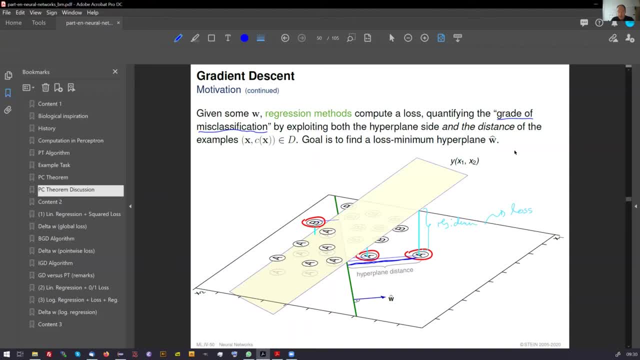 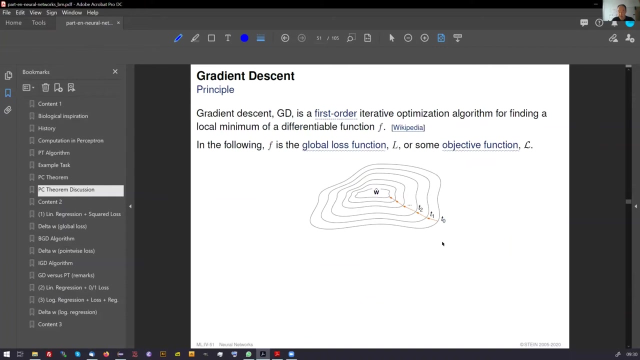 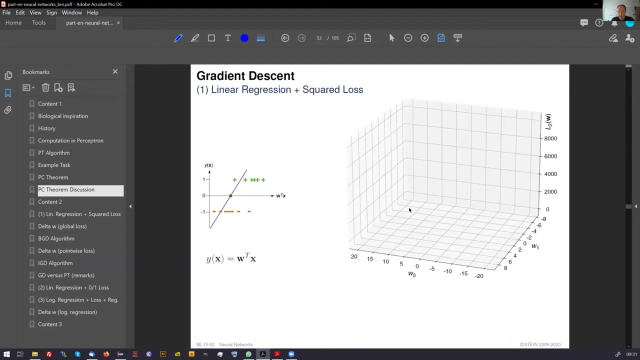 which is not high, but because of its robustness and simplicity it is usually used. Gradient descent wants to get this optimum W value and computes now the loss for all possibilities- You have seen this here- All possibilities of weight combinations here as one. And this, this loss curve or hull, is convex, that means by a. 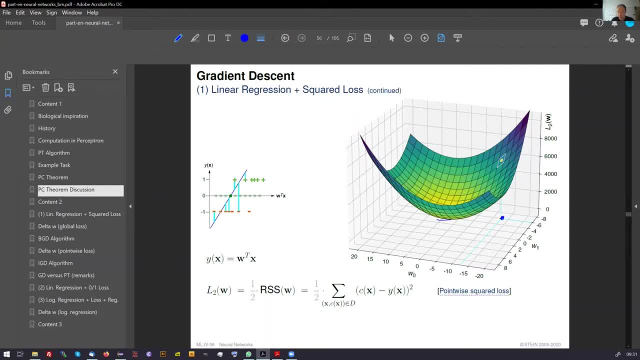 greedy algorithm or hill climbing, a gradient descent, describe all the same, namely that algebraic structure is a matlude, or this is the situation we can find the optimal. This convex situation will go loss if you go to more complex architectures, and this will lead to our second answer. but for the 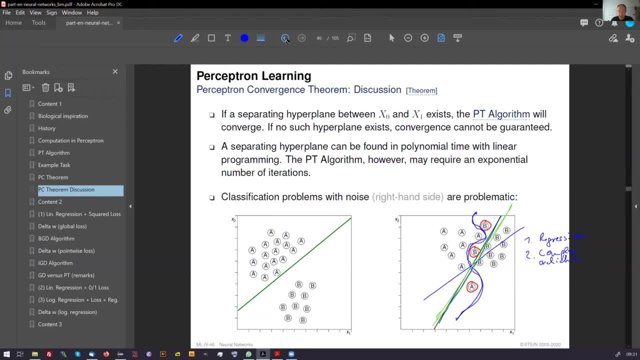 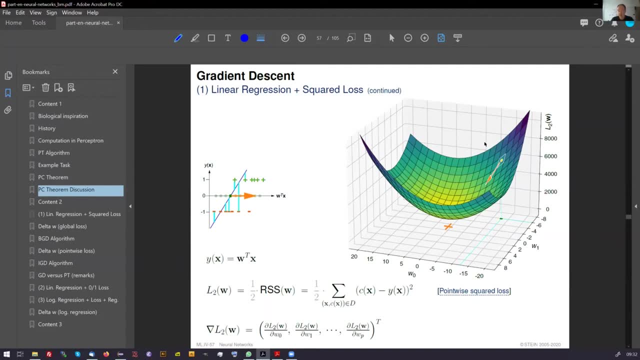 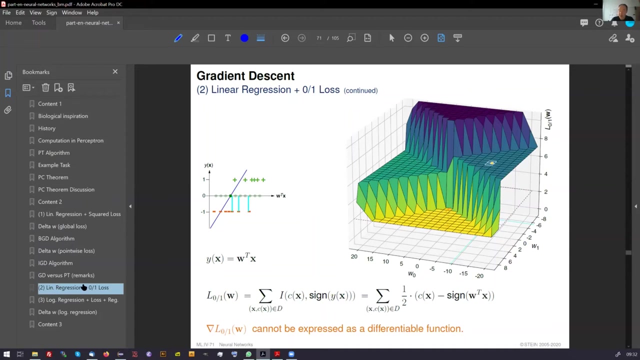 moment. you should see that this gradient descent and convex optimization, we can find the optimal. we have presented a few examples for this, namely the 0-1 loss here which cannot exploit it in gradient descent because we don't know how to move here. and we have also shown a 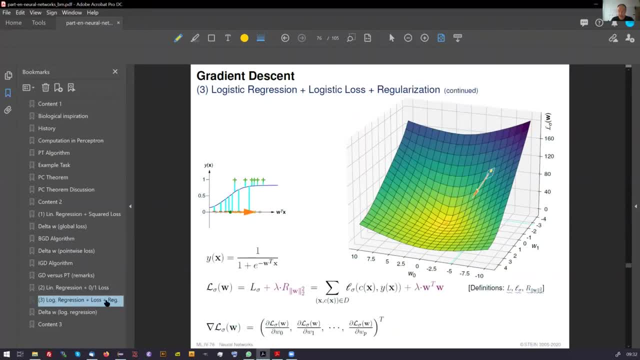 pretty advanced example of this. So it is a pretty advanced gradient descent where we apply the logistic loss and the popularization. What we have changed in the slides compared to last week. we have organized them a bit more logically from the story and you get first presented the classical linear regression. 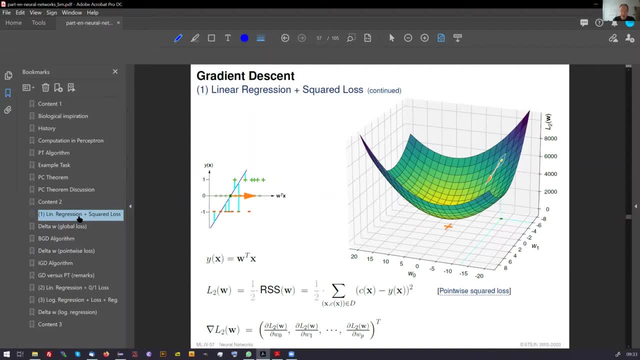 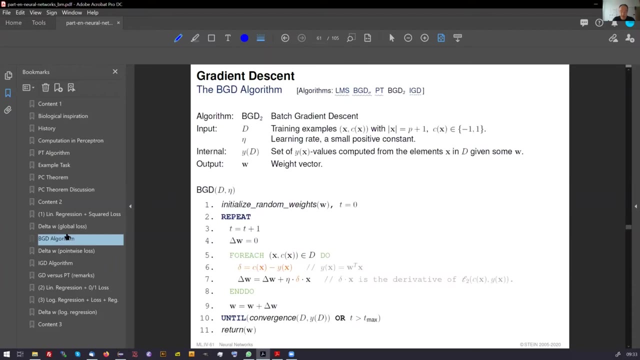 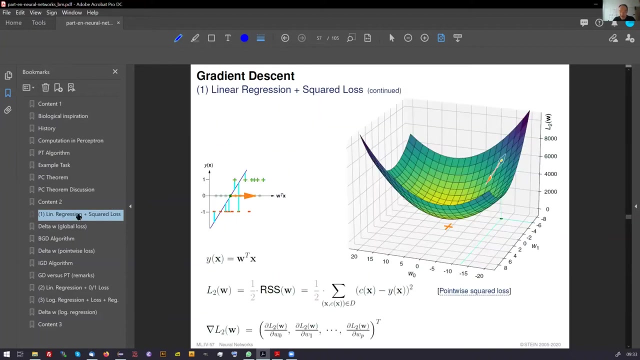 which we solve with gradient descent and not with the pseudo inverse. We show you how we develop the gradient descent method which leads to the edge gradient descent algorithm And around these slides we stopped last week. Gradient descent is effective. sorry, I go here if all examples. 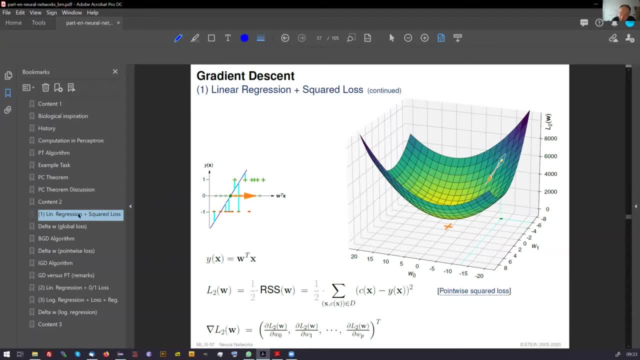 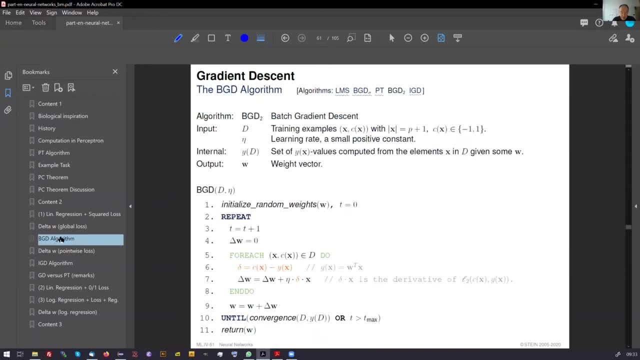 are analyzed to compute this gradient. here We call this batch gradient computation. You see that we have a loop Which looks at all examples, computes the error or the distance or the delta of all examples and adds them. The information that is provided to the algorithm is maximal. 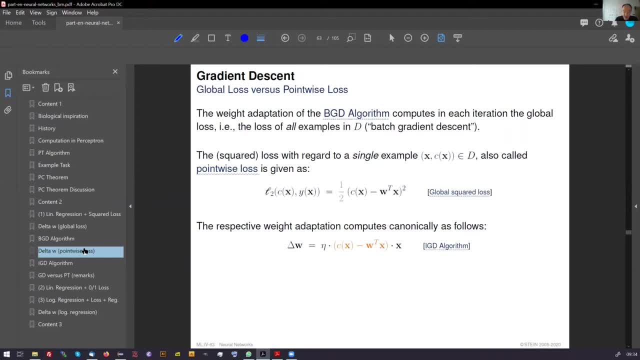 I tell this because this computation of the global loss- it means all examples in D- is not necessary. It gives us the best information but quite often the people use only a local loss, point-wise loss, by considering one example in isolation: The update rule. 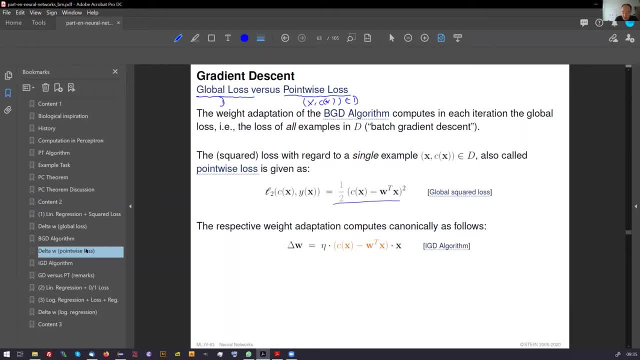 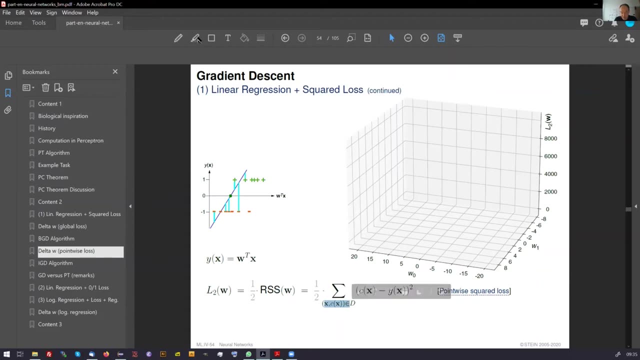 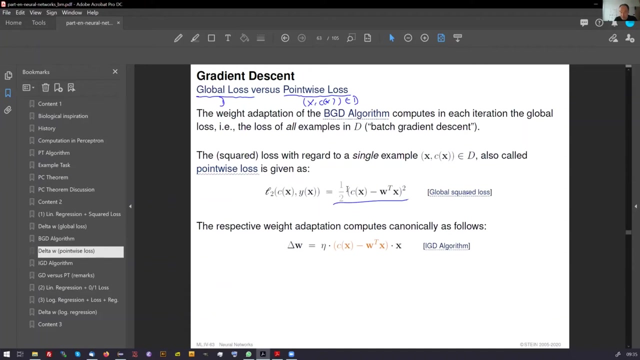 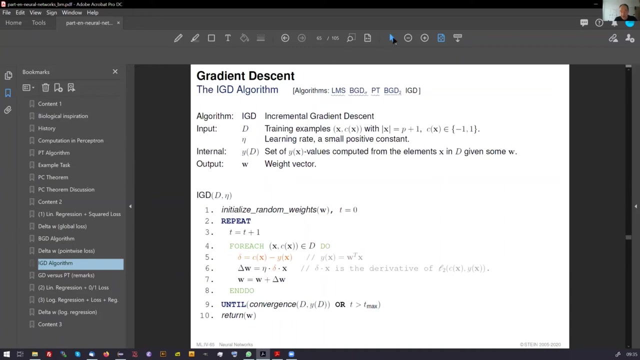 then is simpler, in that we don't see the sum anymore, which you see here, But only the delta of a single example. The algorithm which exploits one example after the other without accumulating the deltas is called incremental gradient descent. And if you jump between these two algorithms, the batch and the incremental gradient descent- 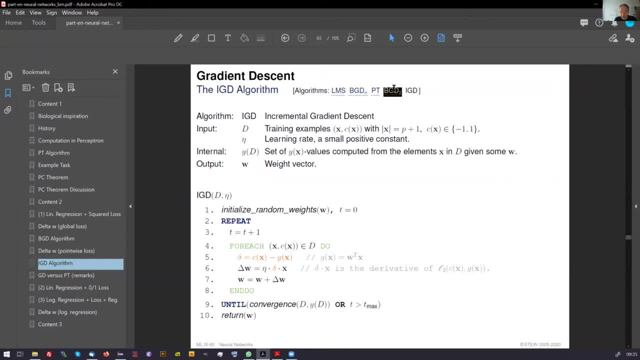 and if you jump between these two algorithms, the batch and the incremental gradient descent, you can do this here, You see, the difference is that the loop between all examples is here. You can do this here, You see. the difference is that the loop between all examples is here. 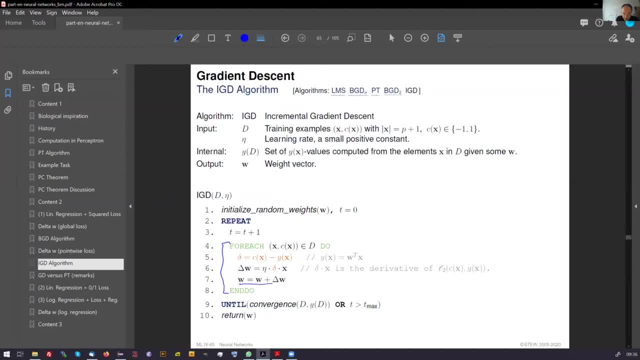 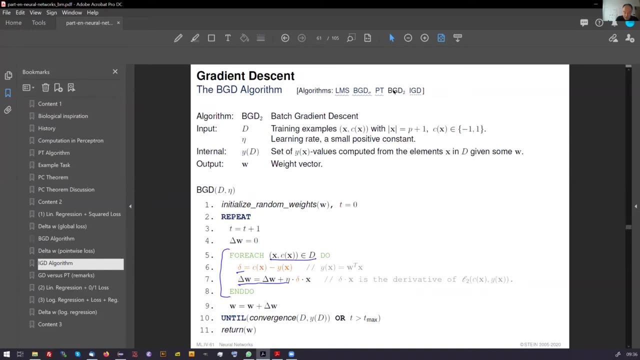 And we have an update of the weight vector for each example. in the incremental gradient descent and in the batch gradient descent, We first accumulate or differences and then do the update or differences and then do the update. If you are working with extremely large data sets, it makes sense to use this algorithm. 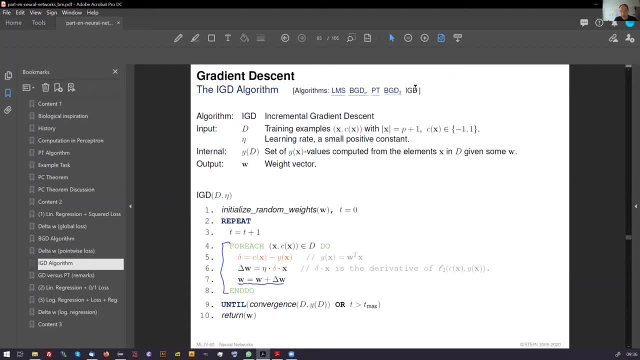 It makes also sense if you have knowledge about how to select framing examples. And this incremental gradient descent or a variant of the rustic gradient descent And this incremental gradient descent or a variant of the rustic gradient descent. gradient descent is your friend if you want to do smart updates within really large datasets. 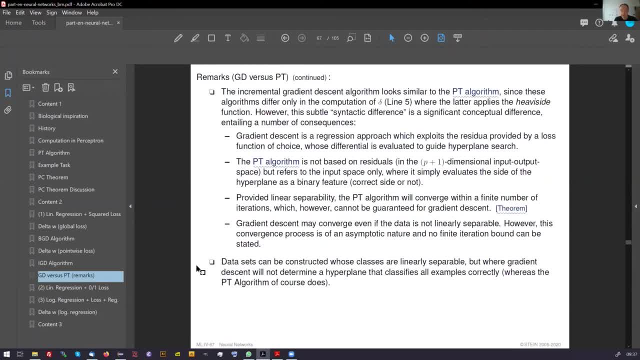 I have provided a short discussion about the difference between the perceptron algorithm and the gradient descent, and the most important point is here. I mentioned it already: the perceptron works only on the input space, while the gradient descent works on the input output space. 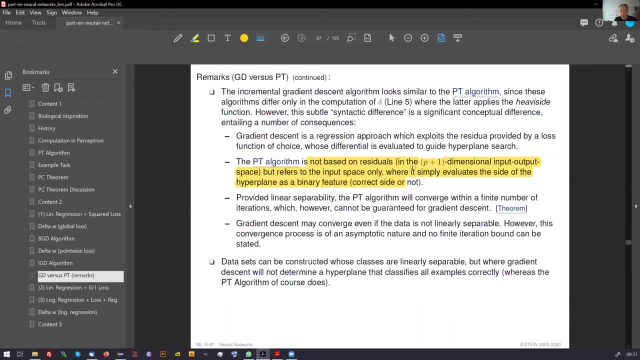 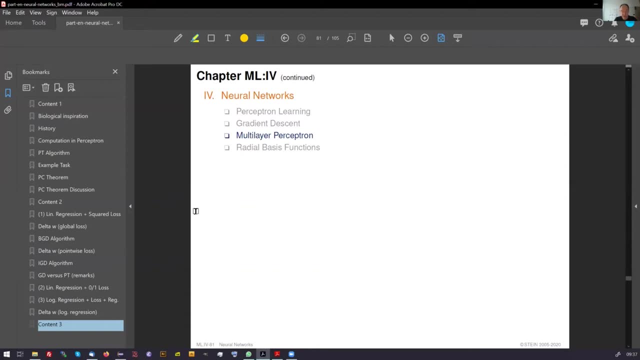 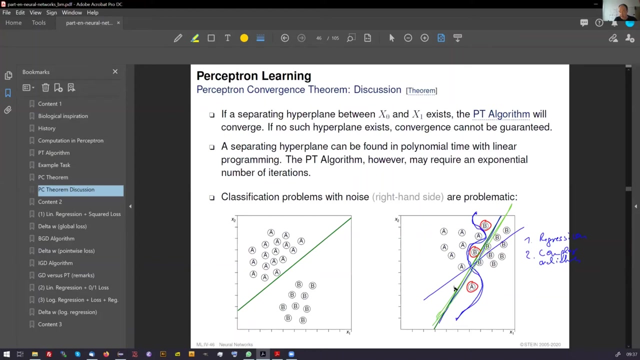 There are also issues with regard to convergence, but for the moment they are not interesting for us. I will now come to the second answer that can be given in this situation, which I showed you here. We can accept misclassified examples, compute a loss, for instance, with regression and gradient. 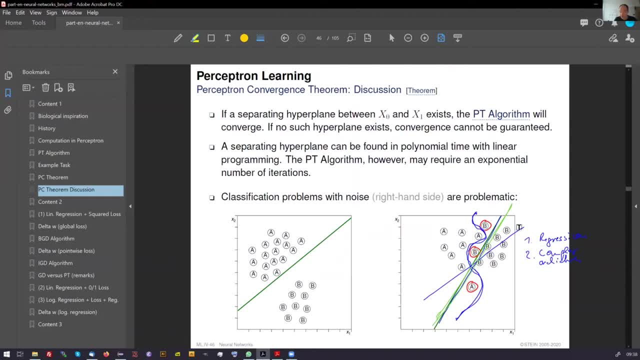 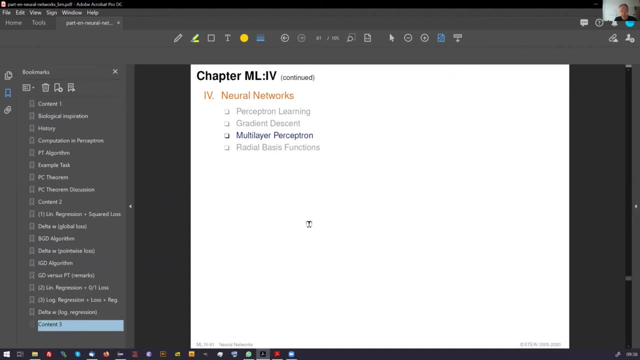 descent. but we can also think about to develop more complex separating planes. This will lead us to the multi-layer perceptron. A note on this: We first define formally what linear separability means. We are given two feature sets and we call them linearly separable if we 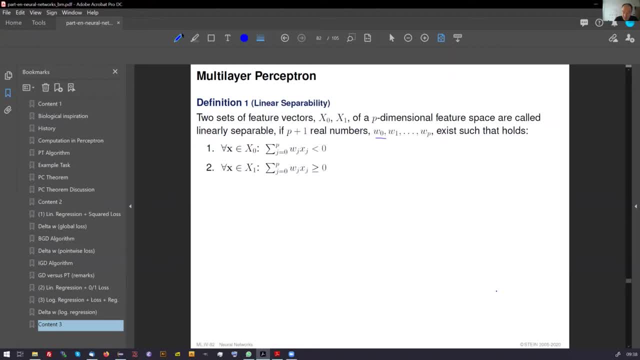 can find a vector which helps us to fulfill these two equations. It's exactly what we saw before In a situation on the right hand side. you see, we are not able to draw a straight line. It will always give an error and, of course, you can use gradient descent. 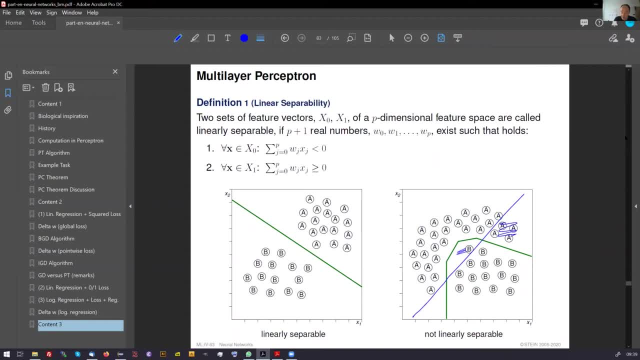 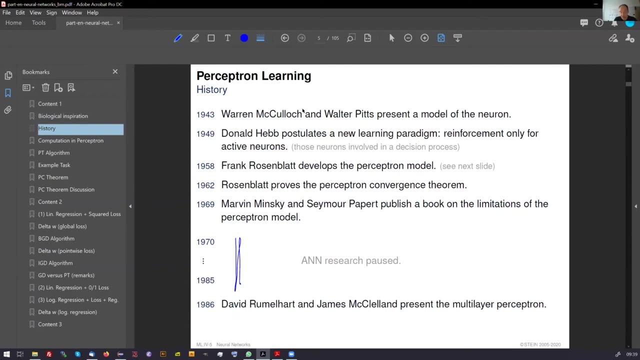 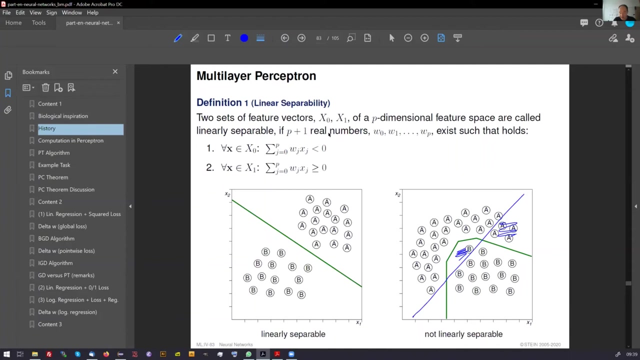 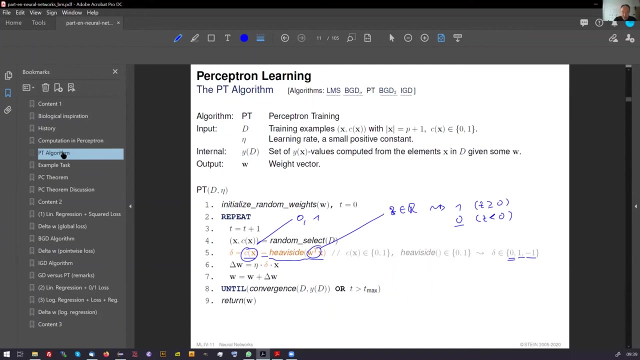 and pay for this here, but the idea it was quickly born that time we can do something more smart here and the first approach to do this failed. if we combine the perceptron like we saw it or like we have it shown here, in several layers, one after the other, we have the problem that we cannot back propagate the error. 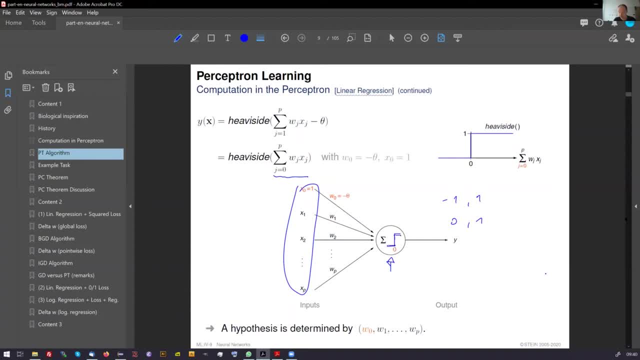 because of this function, the Heaviside function or the sine function. if we use linear regression model here- and Michael, I thought we can do an exercise on this- and combine multiple perceptrons with a linear regression function. the resulting network is the same power as a same low power, like a single perceptron means a combination in. 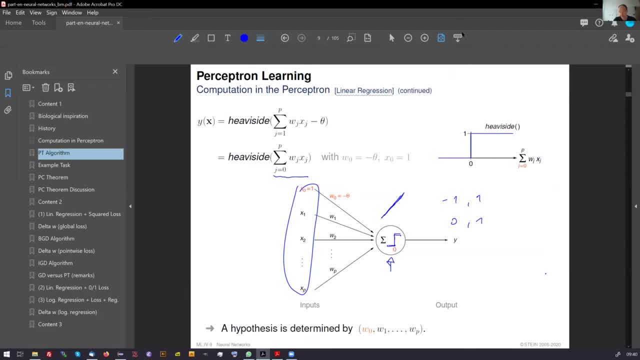 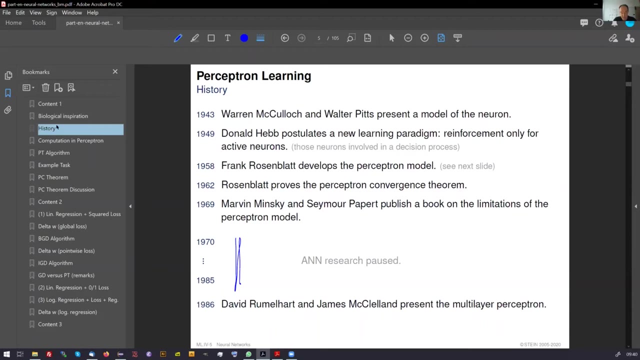 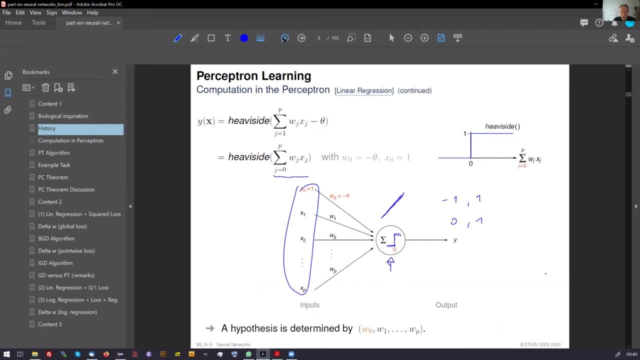 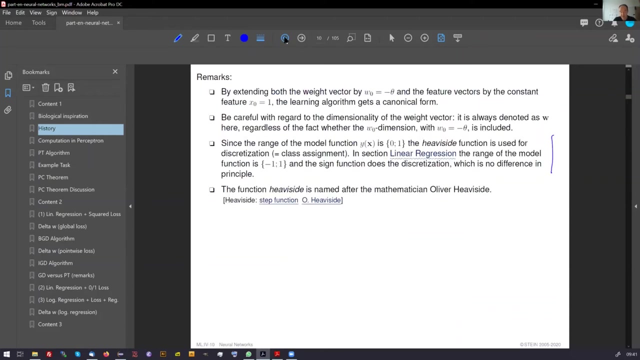 a big network of this regression function does not help you. this is a reason why the people thought it is not possible at all. however, it is not so complicated to find a better solution. but the people didn't. the scientists didn't simply think about this. if it's just a humble experiment, 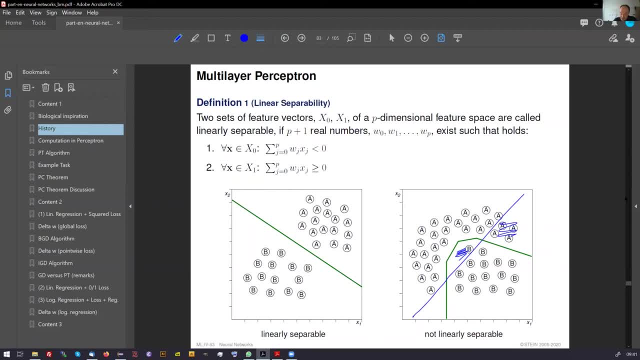 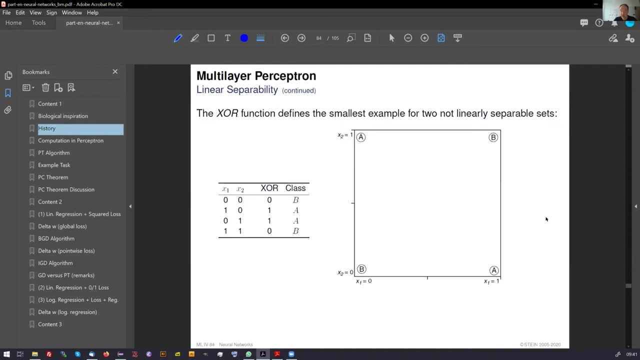 the combination of several perceptrons is nice. the linear regression and it's decision function brings no power, is a Heaviside. function cannot be compact like computer. she cannot be compute the functions inside together and distributed into the. there is to do something different, namely to lose a logistic function. 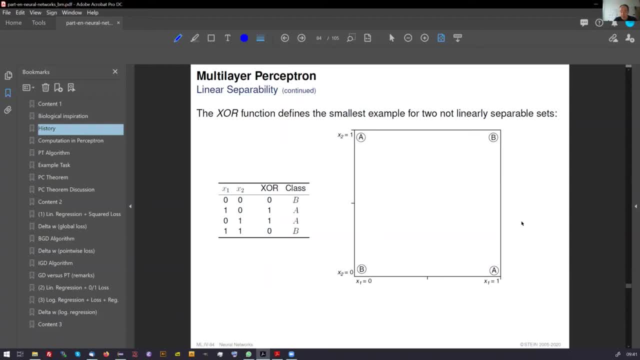 In the book Minsky gave this simple example. We have a setting with four vectors, A and A here with these features, and class B and B here with the other features. And even this simple example cannot be solved with a perceptron. 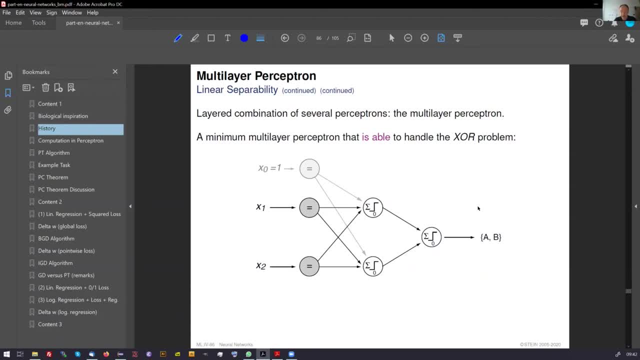 If we combine now three perceptrons like we see here, we can solve this simple decision problem. We have- and this was a problem at that time- no way to find- We can't find- the correct weights to solve this. Yes, a multi-layer perceptron which has the correct weight. 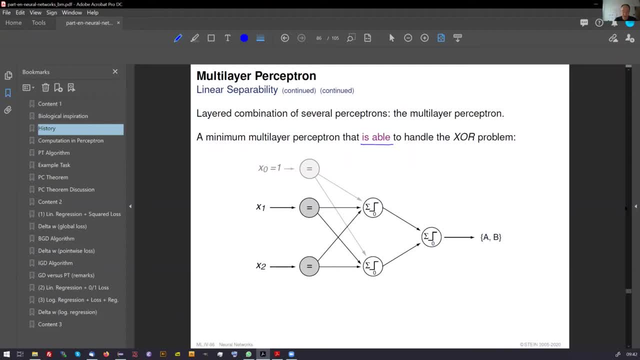 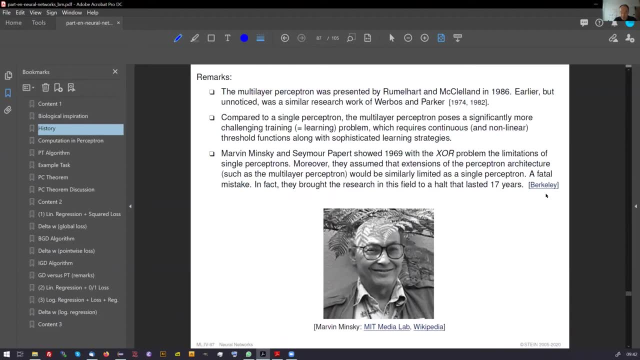 does this decision, but the problem is to get these correct weights. Marvin Minsky, who showed this result, was so influential that the scientists went to new fields and forgot about this, And it took 17 years that I forgot who was it. 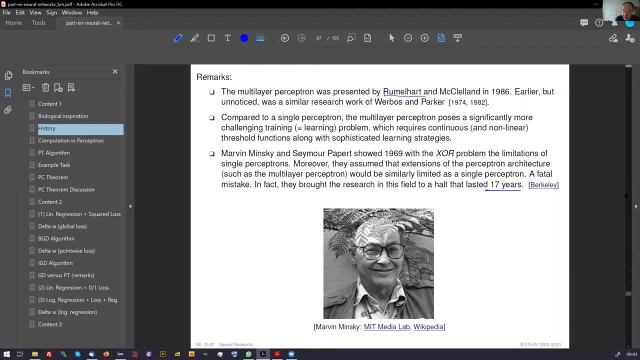 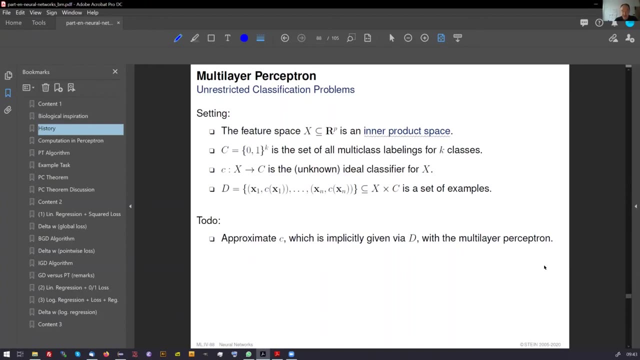 and McClennan- Yes, they were at the end of the 80s- showed that things can be done better. Marvin Minsky was simply wrong. This leads us to the setting which I now call a bit bold: The unrestricted classification setting. 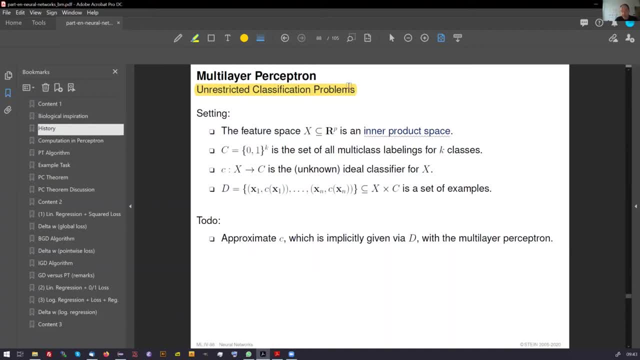 What does this mean? In principle, multi-layer perceptron can solve everything. However, we bring you knowledge about machine learning not to think in this terms. We demonstrate you a large spectrum of algorithms and approaches so that you can search the most suited one for your problem. 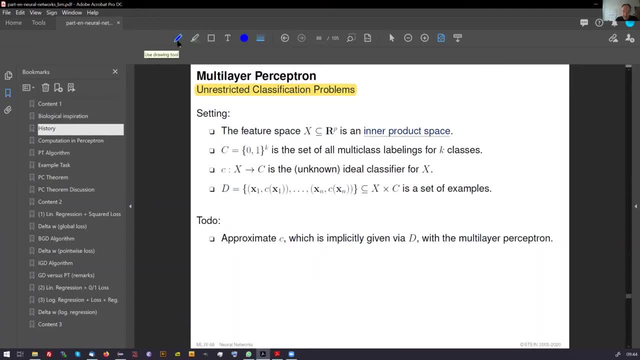 However, the multi-layer perceptron in principle can solve everything. To make this a bit more general, we now do not look only at the binary classification problem, but we look at the classification problem with k classes. In fact, we are thinking of the Cartesian product. 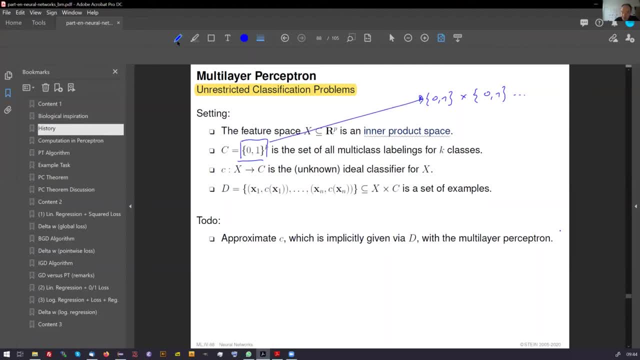 which we call the K-classing algorithm. To find out the class of the k class, we can use a few equations. For example, here we have the k class for k class, And in addition to that we have the k class for k class. 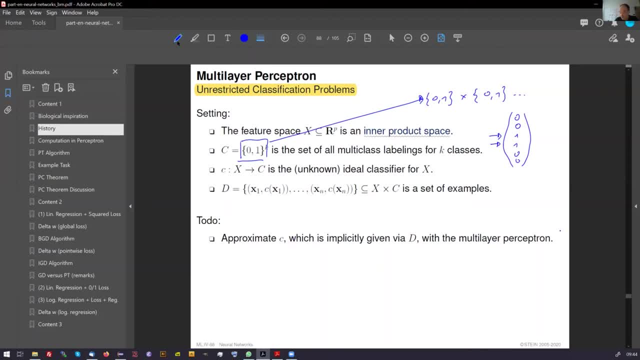 And here the k class is the k class for k class And this is the k class And we can see that k class is a very strong k class because k class is not divided into k class and k class. Here is the number of classes and the most general situation is this one: the set of all mighty class. 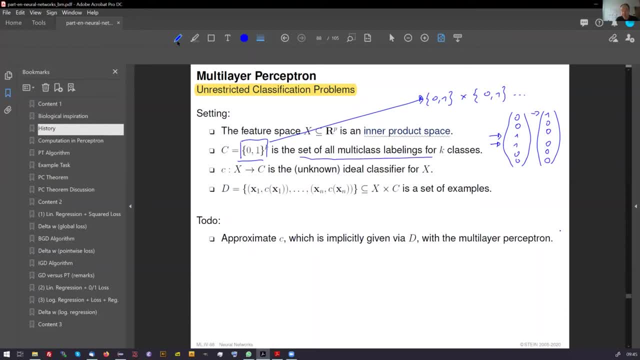 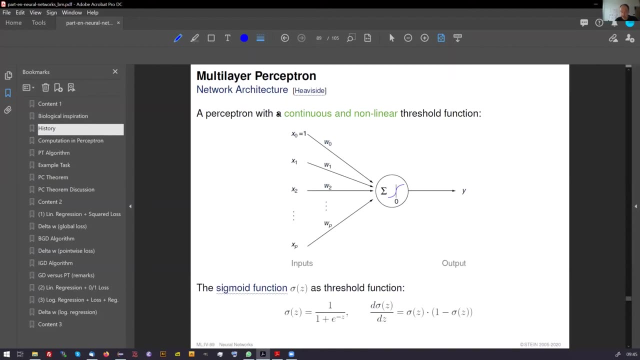 labelings. Except from this, the setting looks pretty much the same, like we had it before, And as a solution we think about the standard perceptron, for which we replace the threshold function, which was a heavy side, now with a sigmoid. The development can be seen here. This is possible for gradient descent, linear. 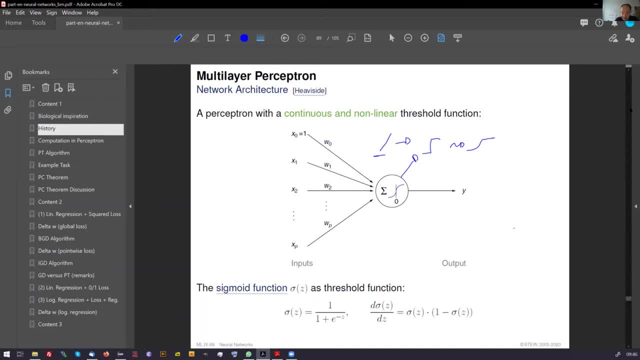 regression. This is- I write this here- gradient descent. This is perceptron training and this is multi-layer perceptron training. Sorry, The sigmoid function is the same as the function which we had in logistic regression. You see it here. We directly give you the derivative. I guess it's an exercise for you to compute it. 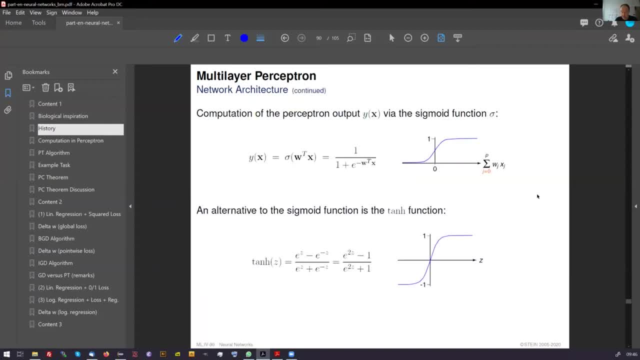 It's not a witchcraft thing And it has this form, No surprise. for the moment, An alternative to the sigmoid function is the tangent-separatist function, which you see here. The most important difference is that the range is from minus one to one. 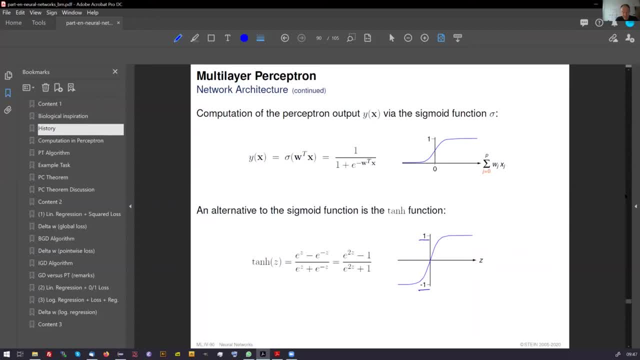 Except from this, there's no big difference. We now build networks which have a more complicated architecture. This is the architecture with which we started: A single layer perceptron, Here now with the sigmoid function. And now we add- you see this here in the so-called hidden layer- other perceptrons. 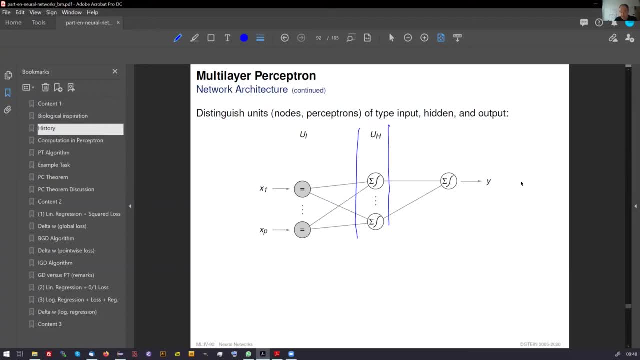 And we combine them in an output layer, And for each class we can use an own perceptron. Other architectures are possible, but with this classical view you can see a lot and you can model nearly everything you need. The variability, the power comes from the weights. 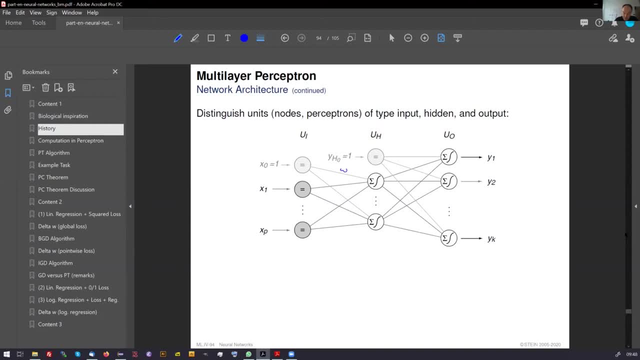 Don't think about the nodes only. We have no weights- I don't write them down here- Which result from the number of inputs and the hidden layer. And we have these weights here And all these weights want to be trained. And we think about examples that we present here. 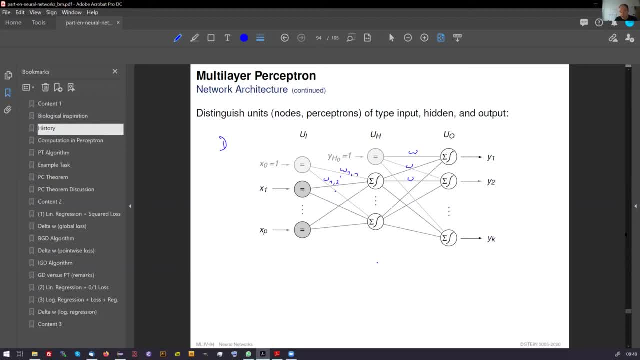 We think about arbitrary, random weights. at the beginning We do a forward propagation, First to the hidden layer, then to the output layer, Then we combine this And we get the Y-vector, which we get is our Z-vector. You see, this is the most complex setting that we can think about. 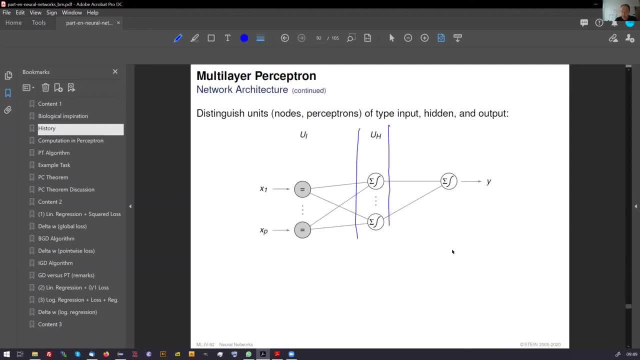 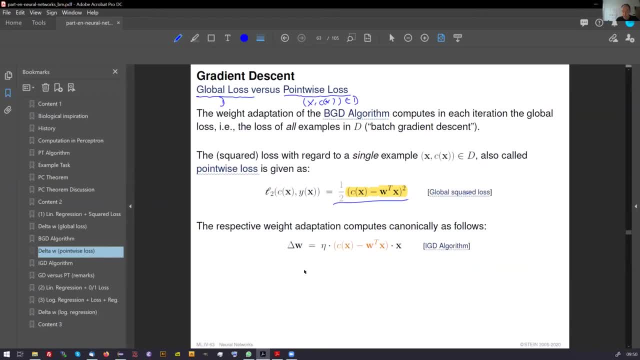 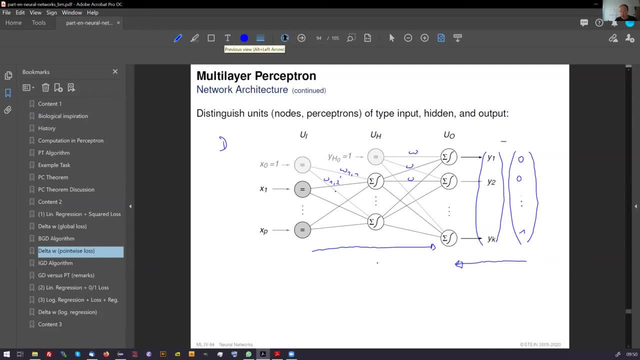 which we learned here to know. Pappert and McClelland found this out. We are preparing the complete derivation of this rule in the back propagation And we'll bring this in the slides as remarks within the next days. For the moment, we want you to understand that we can now build more complicated architectures. 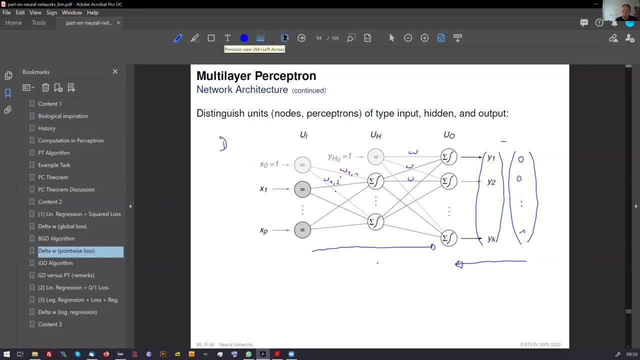 That we need the non-linearity. In the forward propagation, the heavy side would be enough, But for the backward propagation we need a smooth function to back propagate the arrow, And therefore for this we need the sigmoid function. Before I show you the algorithm that we use, 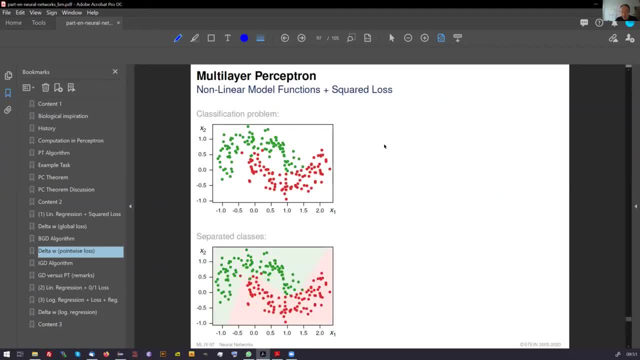 I'd like to show you a few examples of how to do this. Here's an example. Here's an example. Michael developed this from me yesterday. We have a classification problem And it's pretty involved, Although we saw only two dimensions here. 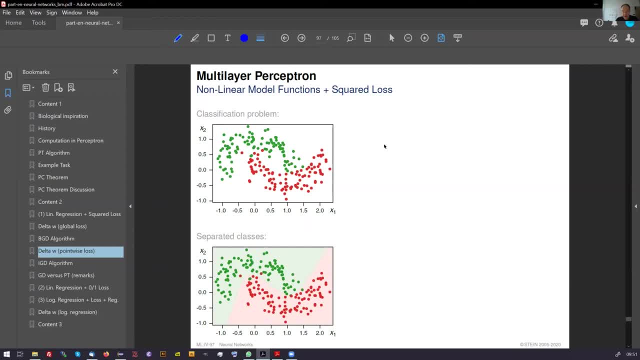 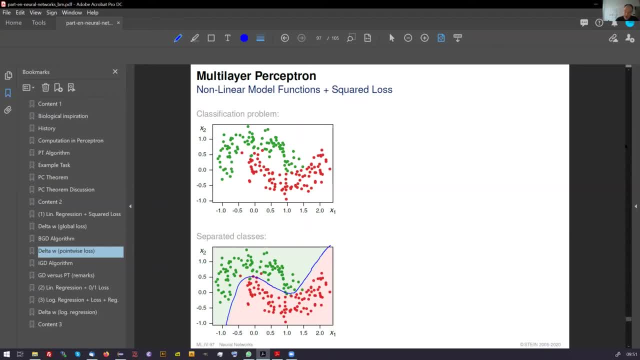 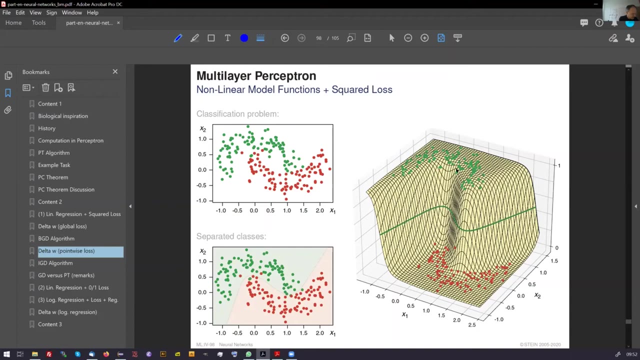 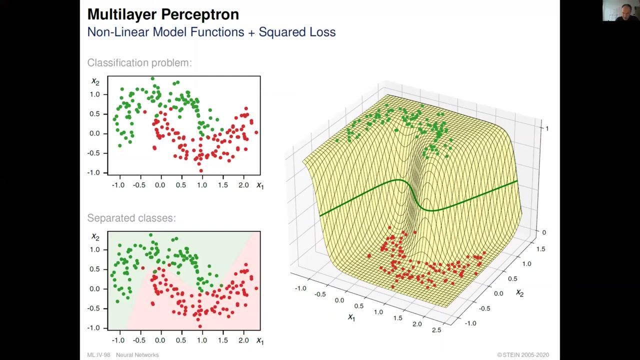 which was learned with a nonlinear model function, which was learned with a nonlinear model function, And this nonlinear model function is shown here on the next slide. Here you can see it a bit better, Here you can see it a bit better. The examples, the positive examples here and the negative examples here, and this decision rule, what we see here, and this was learned with backpropagation and the small network. 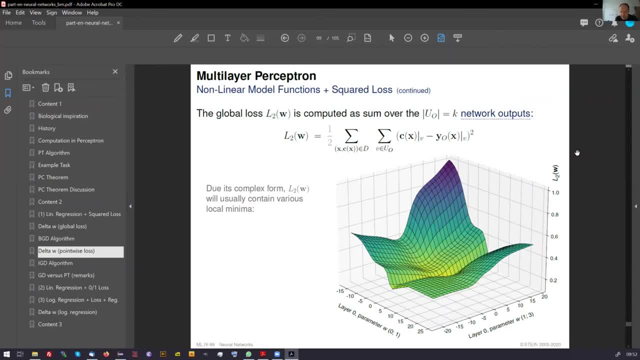 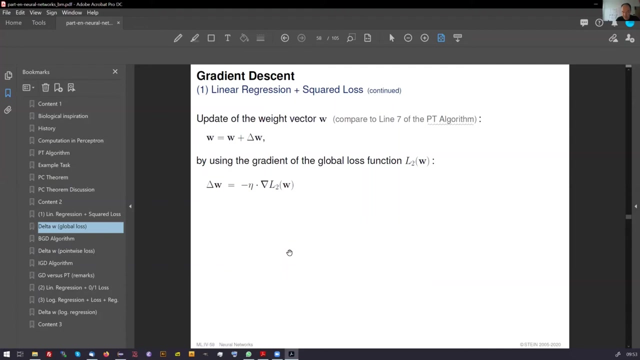 However, here you directly see the problem of this. The global loss now is not a convex function but can be arbitrarily shaped. The global loss which is computed like the global loss before. Sorry, this is in the previous slide- Interesting. 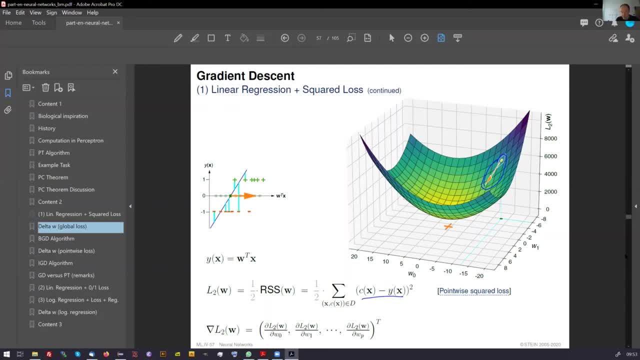 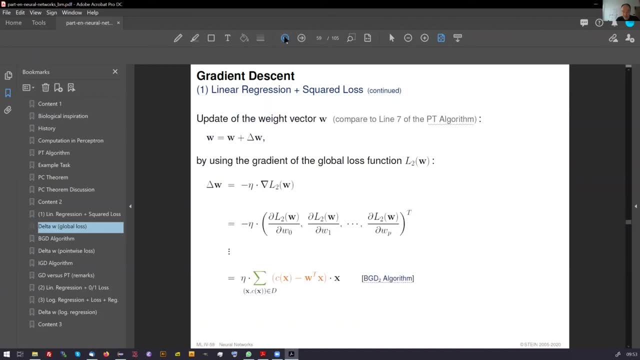 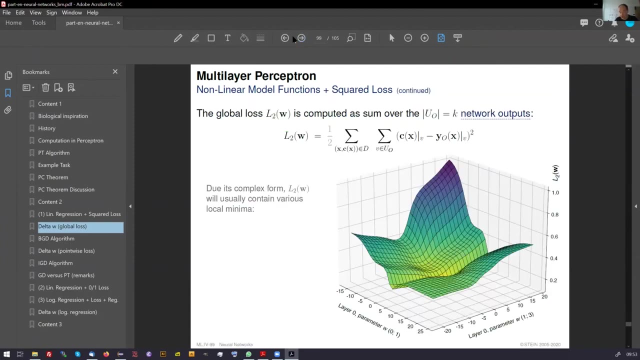 We compute the residual on the square and at them is now not convex anymore, but somehow, In fact for an arbitrary problem, we don't know it at all. That means if you apply such network architectures you have loss The guarantee to find the optimum. 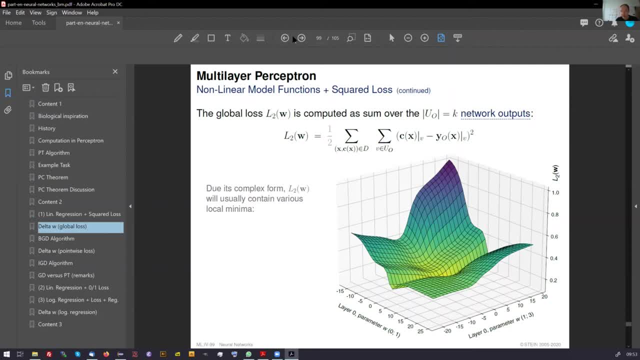 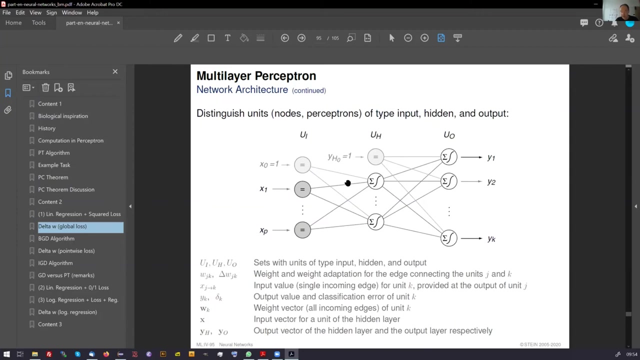 In fact, in many Alchemistic, rules have been developed to find the minimum in such a situation. But, to be honest, there is no. If you go to architectures like this one, The training will always be a problem. I'll give you a few hints you can do. 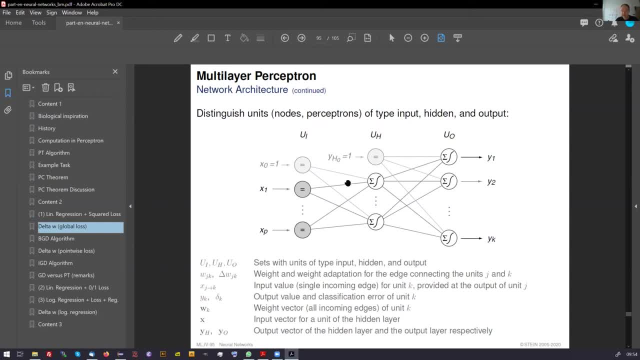 In case you do not have a ceiling anymore, Bring your Electrode refugees. you can, No Qualities, care for the ready policy. doen't give you away easily. there is no law. multiple restarts, pre-trained networks like the deep learning networks. 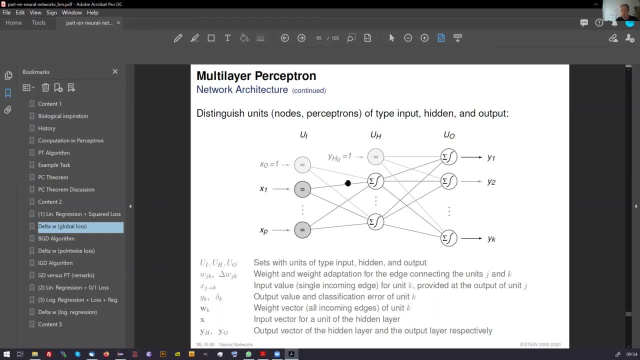 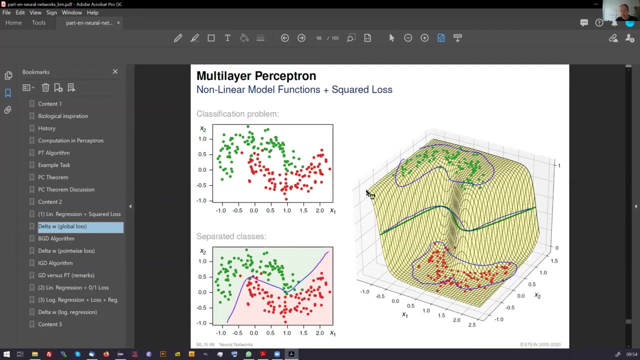 They are pre-trained and want to start with a good point. You can use inertia algorithms to overcome local minima. Many things have been done, But the guarantee that you can argue why a solution is found, Let's use a keyword: explainable AI. This is going. 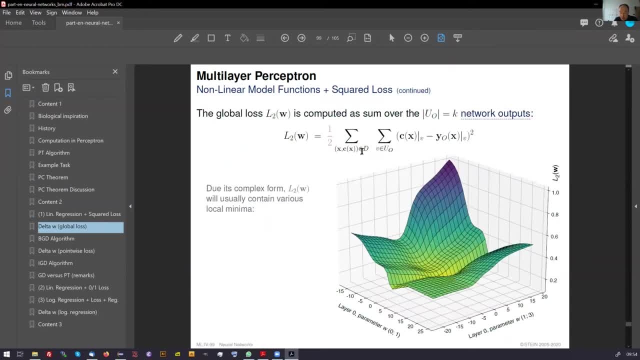 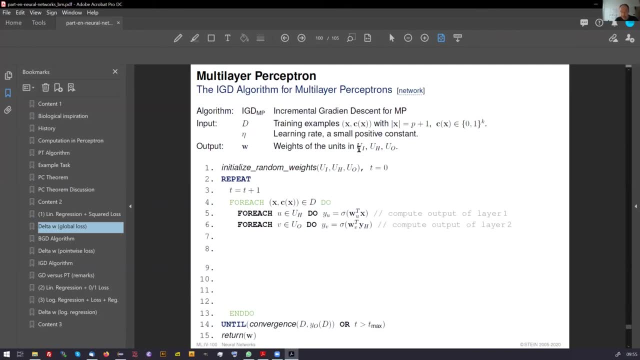 We will develop or show you the algorithm in its classical incremental gradient descent form here now, But we will develop a matrix based algorithm in the next days and also give you this as background material, because we are writing a Scania-based algorithm very similar to the most relevant simpler mathematicals we have had so far. 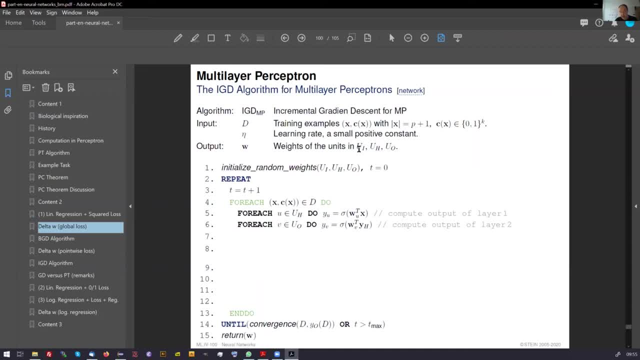 We won't directly go through the framework of deep learning, which argues about matrices and tensors. However, basically, the algorithm runs like follows: You take examples, propagate them to the first layer, propagate the outputs to the second layer, don't worry about the indices. 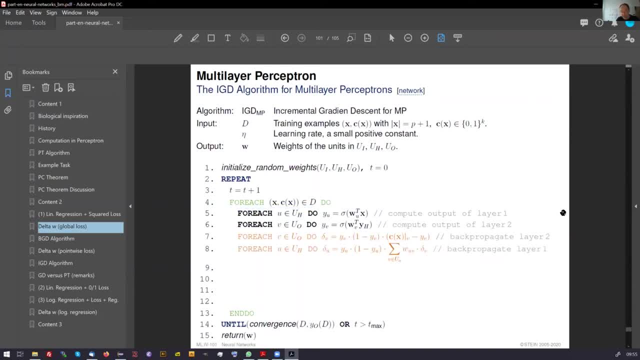 I wanted to show you. it is so standard, easy. Compute the differences at the end, backpropagate them. compute the difference in the middle, backpropagate them and compute some weight update. However, we will rewrite this algorithm in matrix notation. 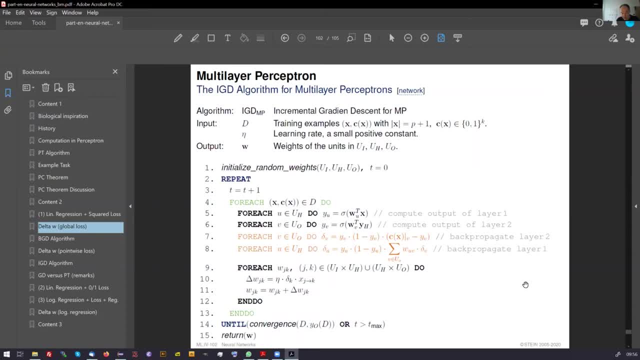 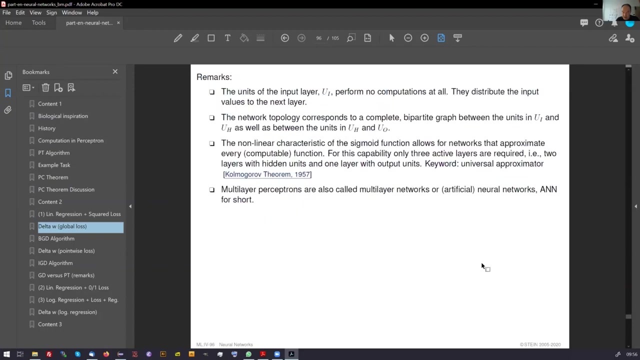 to make it more easier to digest. However, I want to point out, even this algorithm is not complicated for an algorithm that claims to solve, or being able to solve, any classification problem. In this regard, I want to point out the result of Kolmogorov. 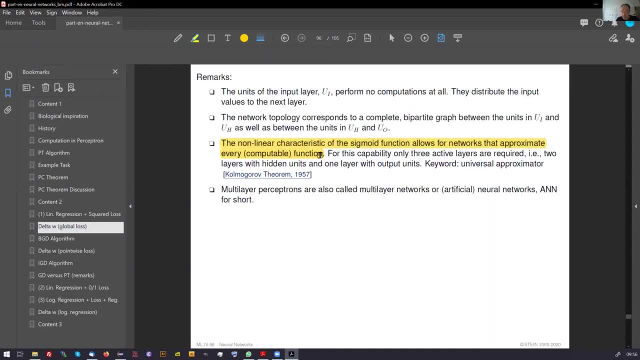 The nonlinear characteristic of the secret function allows for networks that approximate every computable function. Moreover, we do not worry about architectures. He further has proven data Data Only in architecture with three active layers required, with two hidden layers and one layer of output units. 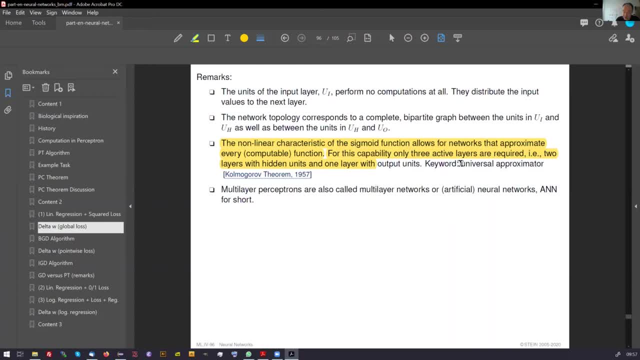 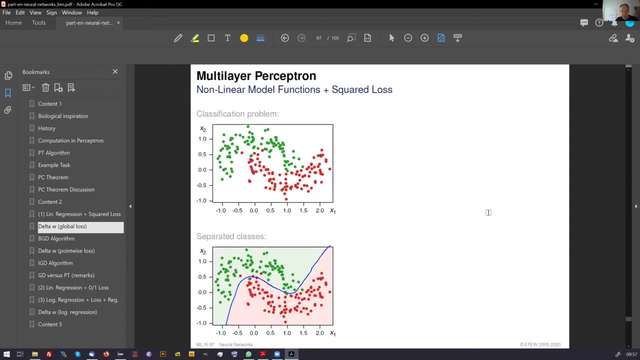 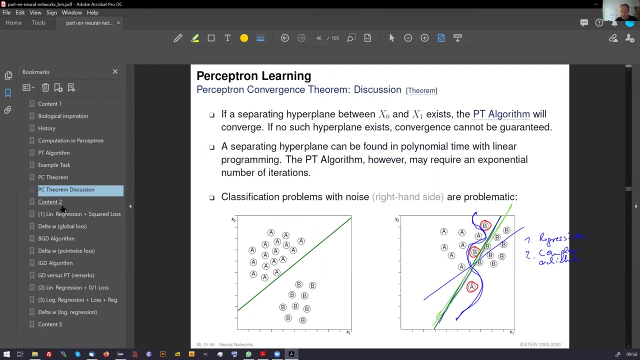 With this architecture, you can program and compute everything in theory. This is more or less the most important message of this reading, Rather a short reading, but with essential insights. I want to recap this: what we did? The perceptron algorithm, although it is very primitive. 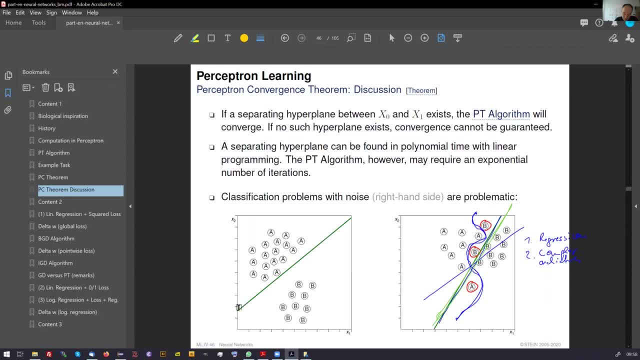 and can solve only such problems. sorry, gave rise to architectures which are able to draw this line. This became possible by switching several of these perceptrons together to a network, but equipped them with a decision function as a threshold function, which is non-linear. 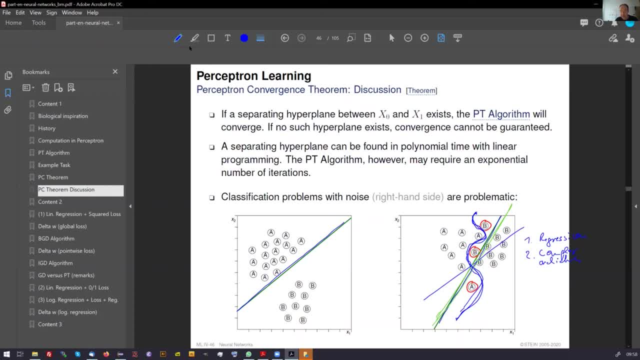 but still differentiable. Non-linearity is essential to get such complex decision lines and differentiability is necessary to do back propagation. If we build such multi-layer perceptrons, we lose the probability, the guarantee of finding the optimal. The loss plane is not convex anymore. 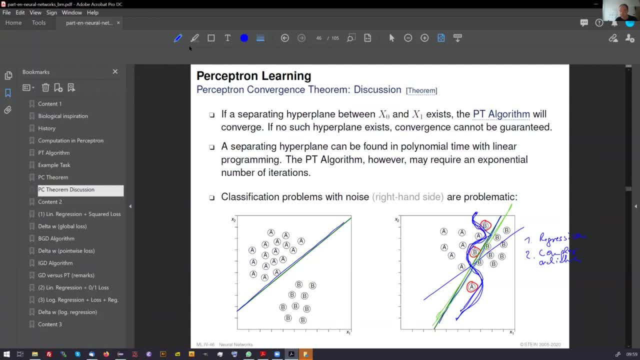 What we win is that we, in theory, are able to approximate any function and that we can solve any classification problem. However, if you have a good understanding of your data, logistic regression with a good regularization term is the most effective you can do. I would say this is enough for today, and what comes next is that we bring matrix or tensor work. 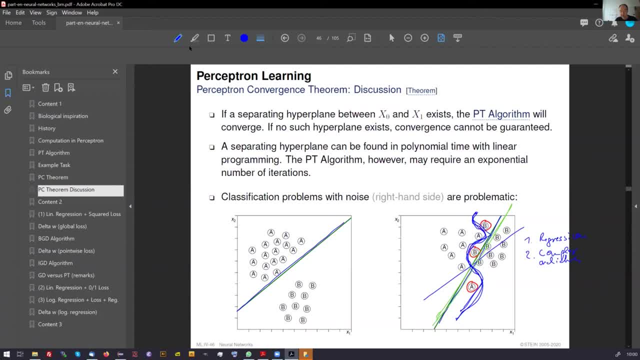 on the matrix- We have two versions of the presented algorithms here- and then go over to a new class of algorithms, namely the support vector machines which measure the distance between hyperplanes and which work completely different than the algorithms which have been seen here, which are all regression based. 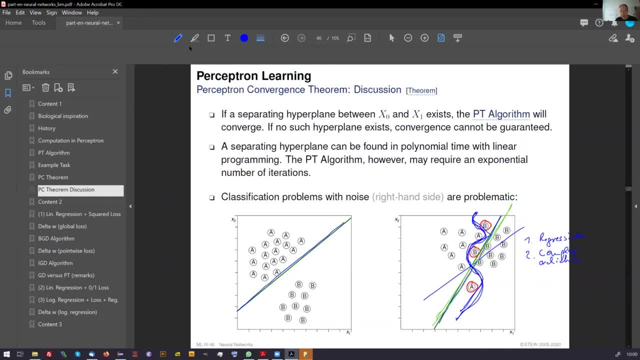 We have presented the multi-layer perceptron and we will show you the connection, which we will pick up at the end of the reading, to so-called deep learning approaches. From my side, that's enough for today, and I can only say a nice goodbye. Thank you for listening and being here and trying to understand what machine learning is about. 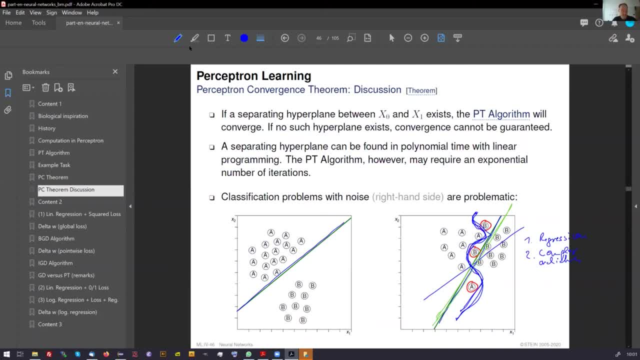 Thank you very much. Thank you, Benno. I have maybe a very short question, which maybe is just a syntax thing. The C function suddenly became bold-faced. Can you give a slide where I can, For example in the algorithm 100, slide 100,. 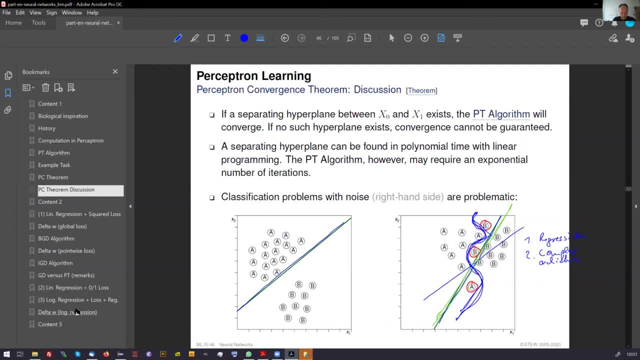 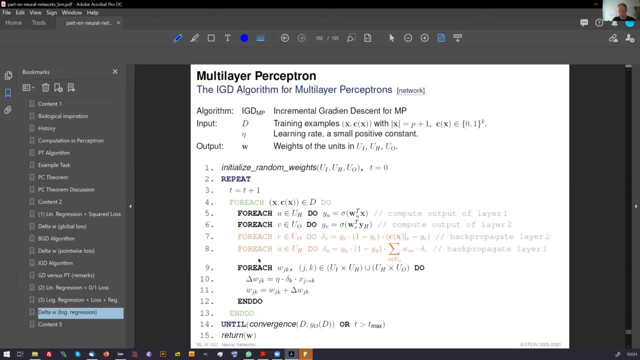 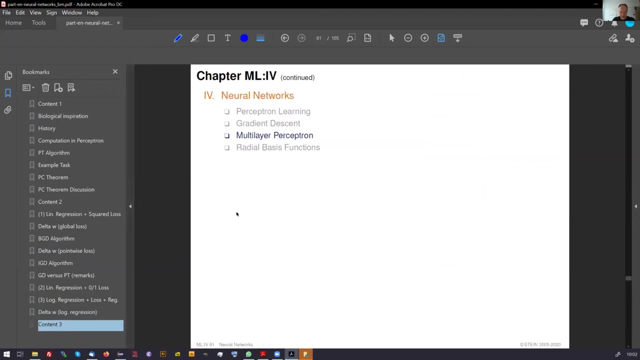 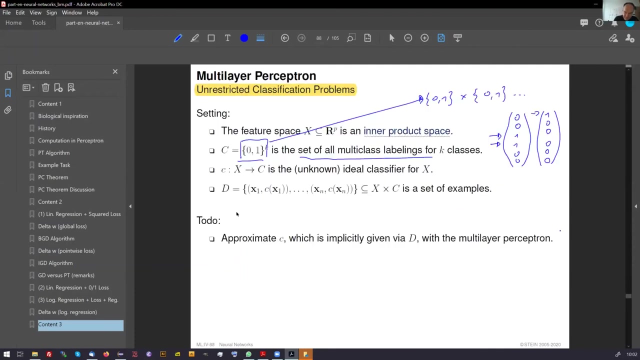 slide 100-2.. Yeah, this is clear. We now map onto this problem. Thank you for asking. We now are in the setting here. It was there. I think I can see here where the map output this vector, namely one hot vector like this, a multiple labeling vector like this: 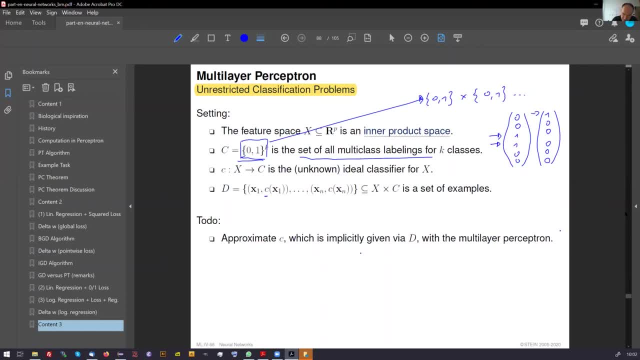 and you point me to an error. In fact, this should be bold here. This was wrong. Thank you for pointing This should be already bold. This should be BOLD. I see, Yeah, because we have a vector of functions here. 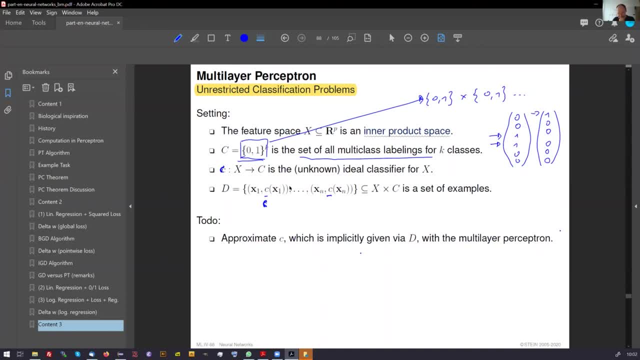 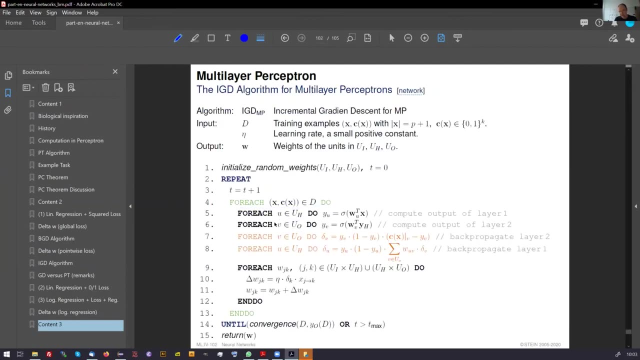 I will correct this, sorry, Thank you. This is Michael suggested to go away from this description which you see here to a matrix description. I liked this description which you see here because a matrix description removes complexity but it is not so complex. 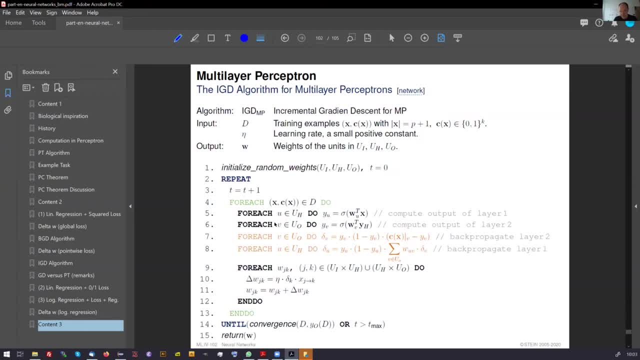 This algorithm, which you see here, can be directly implemented in your language of choice. If you write matrices, this becomes a bit easier, but the implementation behind this has to have this form. But we will change this and then we will also see the vectorized functions. 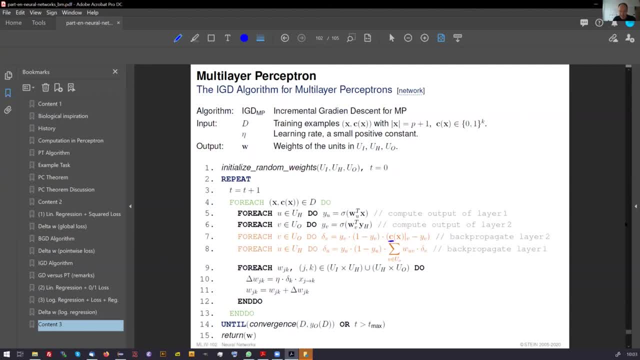 which are mentioned here. Michael, if there are no further questions, you might take over and present insights of the submissions or other hints. how to cope with the algorithms in the environment, the Python environment. Right, yeah, there isn't much planned for today. 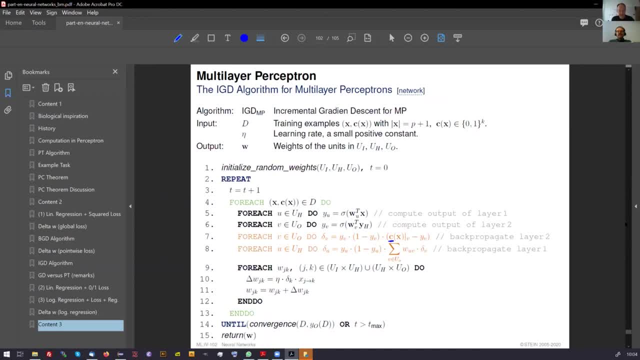 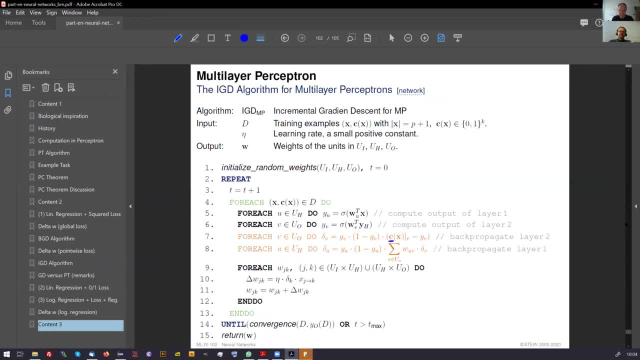 Maybe we extended the deadline for the exercise sheet because a lot of people had trouble finishing on time this time. I guess there was a lot of other coursework going on in parallel that made this a bit difficult. So you still have until tomorrow evening to complete exercise sheet three and sheet four. 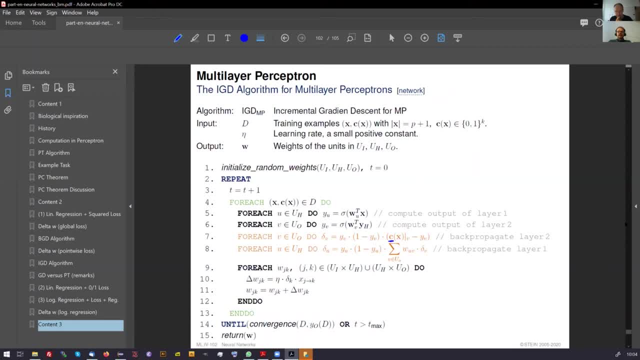 then will be online in the next few days And we will adjust the deadline for that also accordingly. And can you provide me- all the other students- feedback what which things are running well and which are more complicated and not to be loved? that i'm not sure. yet i haven't looked in detail at the submissions. 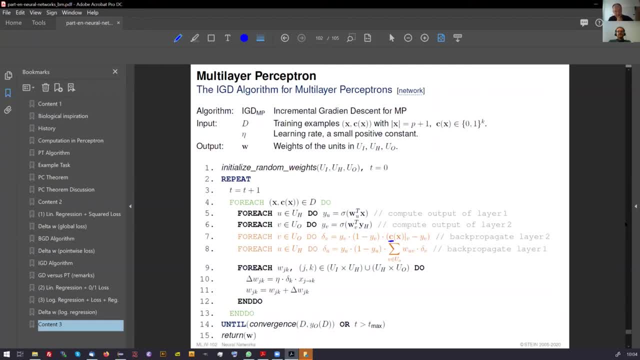 for sheet three, because, well, not all of them are in yet. i suppose is there a tendency to has a program or to answer also the theoretical questions that we give. well, of course they have to do both and are doing both. so, yeah, okay, i guess, i guess for the leipzig side we might. 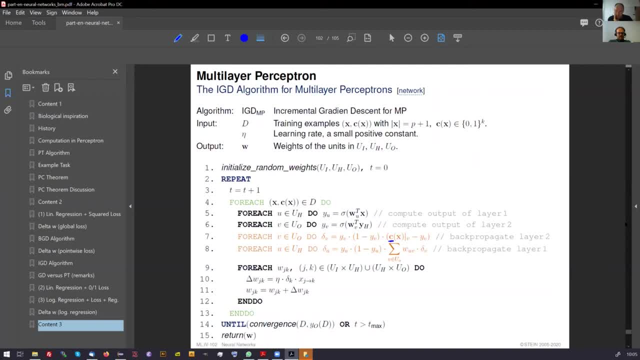 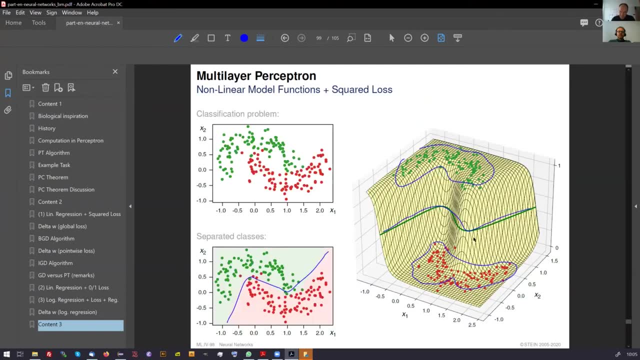 get to get a picture with regards to where people stand, because there is that's not mandatory to submit. yeah, right, that might probably be this, maybe just for just to see. yeah, i will definitely need some help reviewing them then. yeah, the tas can take a brief look. we don't have to look at everything, i guess. 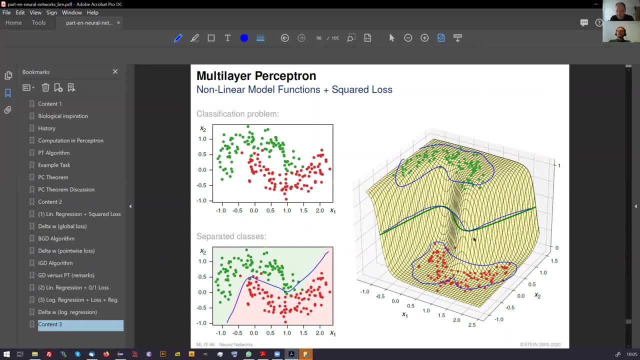 just to get an impression. perhaps possibly you wonder at the students why we explain how the algorithms work and where they were developed from. you will find out if you're working for a company. it is not the first job for you to provide a solution. this is the first step, but it's not the primary job. the primary job is to explain why the solution. 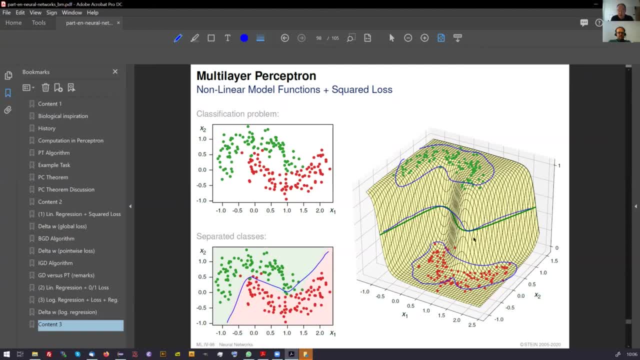 works. this is the hard part: providing a solution without explaining why it could work and where it could fail is not worth much, and this is what we want to explain and bring to you: why does it work? until when does it work and when can it not work? 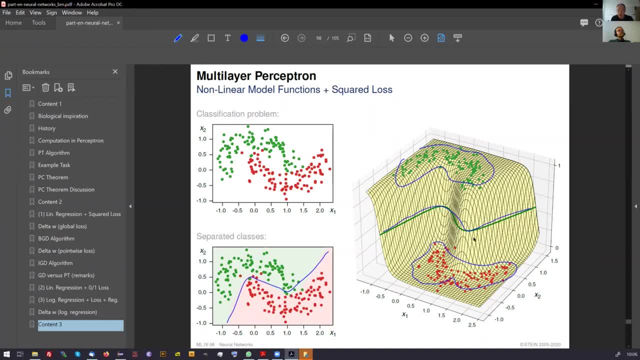 anymore. for instance, you should know when you are in a convex situation. you can guarantee to find the optimum. you should know what you have to pay, namely a weaker or simpler decision line, but you find the optimum for this and this connects to the third and fourth reading. this introduces 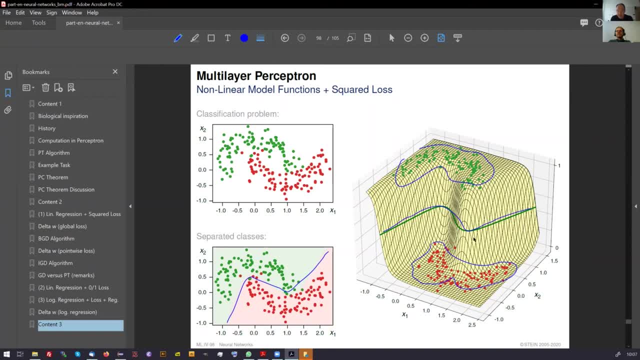 a high bias. you are simple with regard to the decision mode. if you want to be very strong with regard to the decision role, like here, we apply arbitrary non-linear model functions, so you might think about it. you can promise everything but the variants in training. these are so complex that it might be high risk to go in this direction and you have to well justify. 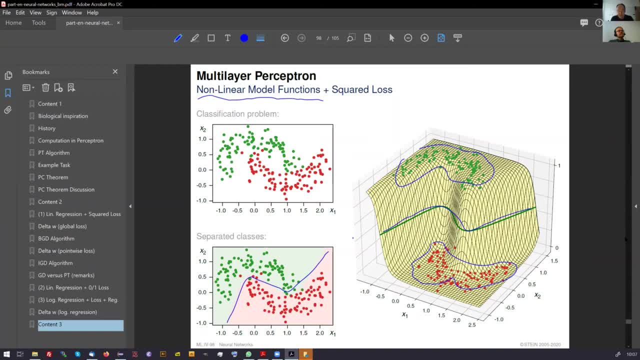 the choice of the network. if you have plenty, much of data, plenty much of time, plenty much of computing power, this is a great choice. until i present one, and nowadays there are situations where we have this: we might train on the internet archive, we might have super computed our hand and we